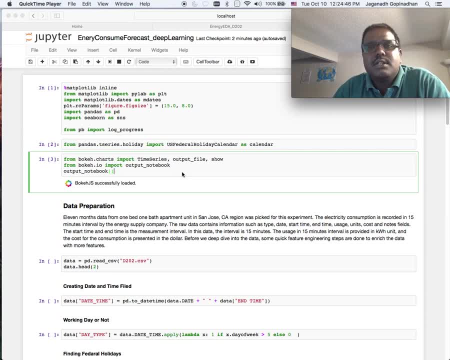 But the problem with energy consumption is that, or electricity in the world, is that there is always increased demand and there is a lack in the supply. So always energy companies. what they are trying to do is that they look into the future demand and try to procure or increase or decrease their supply or the production. 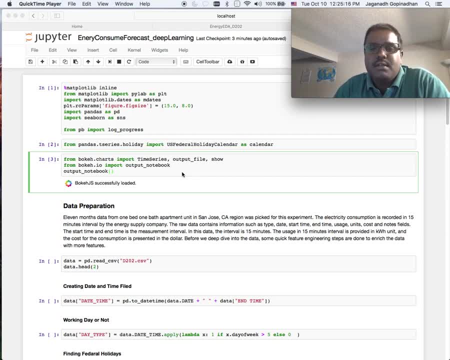 Depending upon the emerging trends and needs. So that is being affected by different conditions such as the weather or some of the festivals, etc. etc. So many factors may be affecting Africa. So I am just taking a smaller sized or a reduced version of that electricity consumption forecasting. 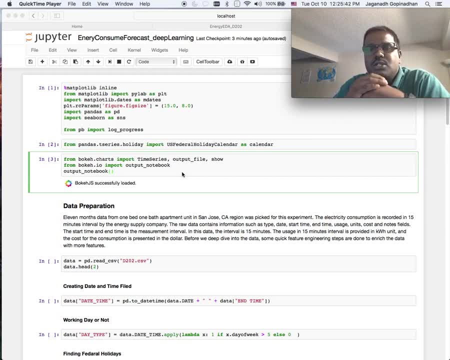 What I mean by, or the meaning of, reducing is that I just downloaded. I just downloaded The energy consumption- the historic energy consumption- for my own apartment unit in San Jose, and I downloaded around 10 months worth of my energy consumption details from my energy. 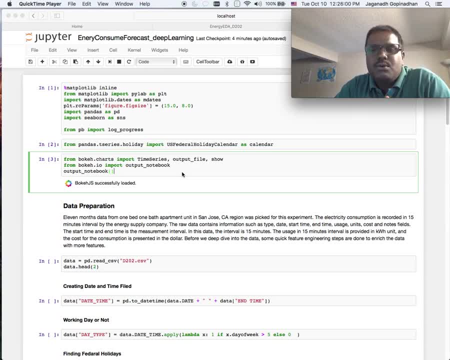 supplier, PG&E, and I am trying to build a model to forecast what will be my energy consumption. So that is what the overall problem statement Which we are going to cover in this tutorial. So let us look into the key attributes of the data. 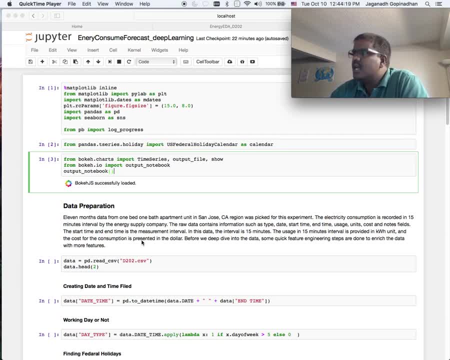 So the data contains information such as the start time and time of conception. So the start time and the difference between the start time and time will be something like a 15 minutes interval, as PG&E records the energy consumption in 15 minutes interval And the conception is recorded in kilowatts. 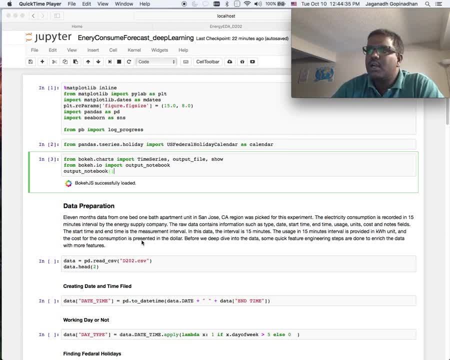 So that is what we are going to talk about in this tutorial. So let us look into the key attributes of the data. kilowatt and the cost associated with the kilowatt hour consumption is being also recorded there in dollar values, And that is pretty much the useful attributes in the data. 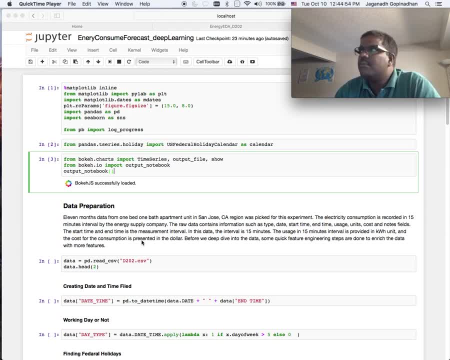 So now let's start doing everything in a pretty hands-on mode. So I'm using Python as my tool chain, I'll be using a skillet and Keras as my primary tool chain for building the deep learning model and then the conventional model. I'm using Pandas for basically the data manipulation, the time series, data manipulation, data loading. 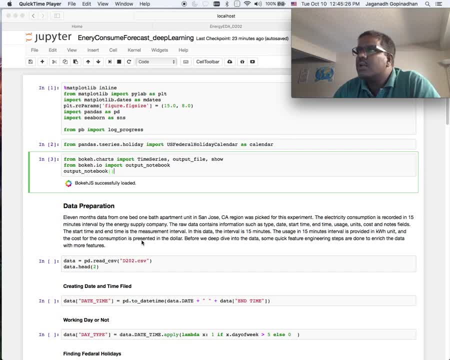 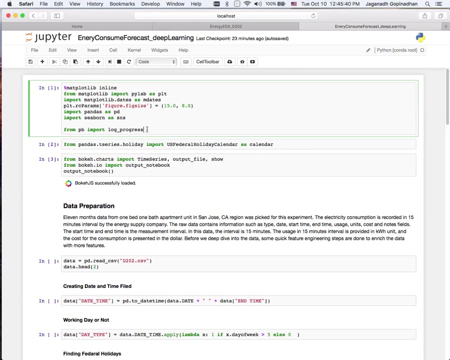 and data preparation etc. And the entire tutorial is built on an API. So if you're interested in how I built my EDU Python notebook, which is a convenient way to create reproducible research here, So let's start from the very beginning of my EDU Python notebook. 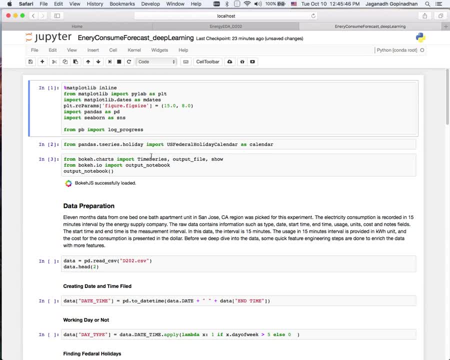 Here. what I am doing is I am just importing all my required libraries, such as MyPlotTradE Pandas, And I am just importing the US Incredible Federal Calendar from the Pandas time series library And I'm importing the Pandas file and I am just importing the PDF file. 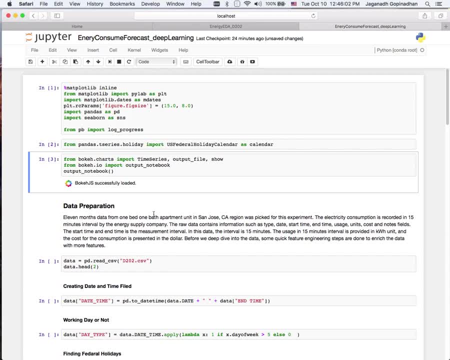 And I am just importing the PDF file. And I'm just importing the PDF file And I'm simply doing this and then I'm just using a bit of the API and I'm just importing bokeh library for interactive exploration of the data and i've just saved the data as d202. 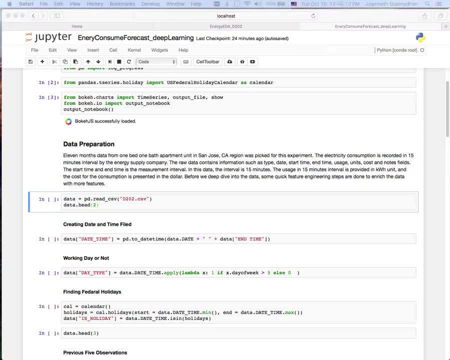 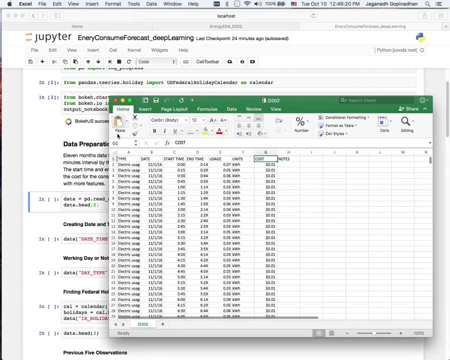 dot csv in in my computer so that's a csv file. so this is a quick view of the csv file which says that the the csv contains type, the header, type, date, starting and time. you said unit, cost and nodes. basically the nodes field has nothing in it. okay, the type is required. uh, written as electric. 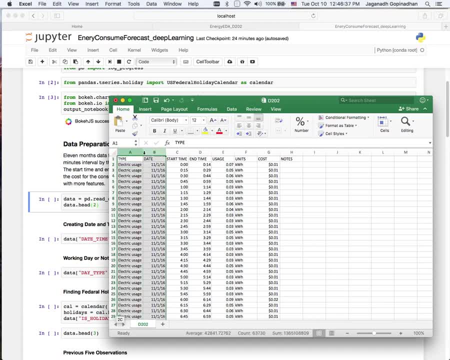 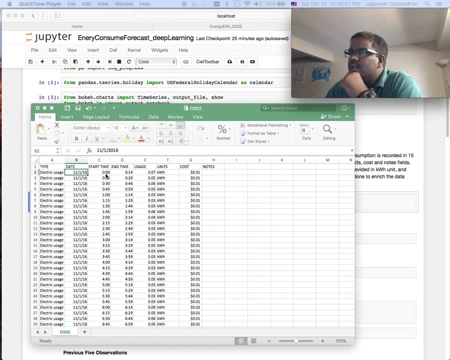 usage. yeah, i don't have any other, any other subscription for pg and this is very obvious, that only electric usage is there, and then i'm having something called dead here and uh, then then the start time is recorded here, then the end time, uh, and how much electricity i use. so 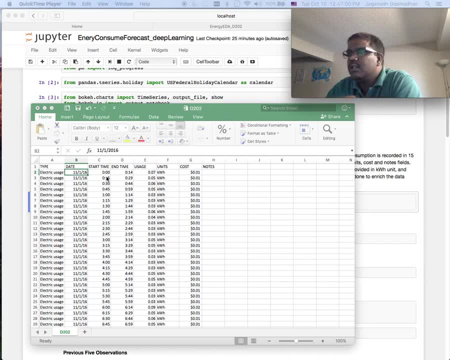 it's means that on 11th uh 11 1 2016, i used uh 0.07 kilowatts in the first 15 minutes and i have to pay like almost 0.1 cent as a cost for the electricity. so this entire data is starting from 11 1 2016. 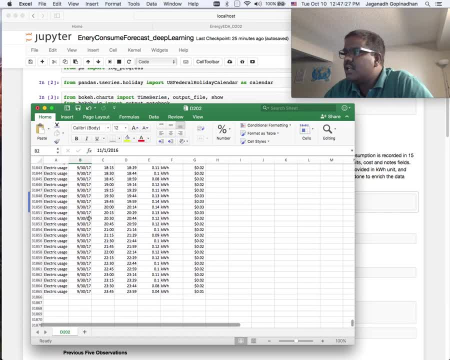 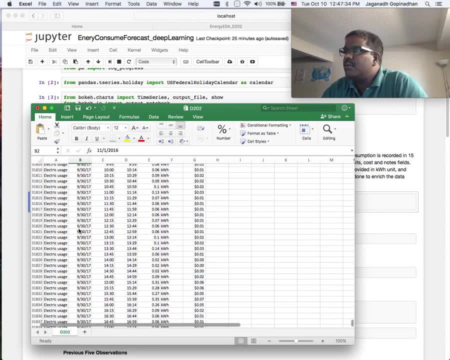 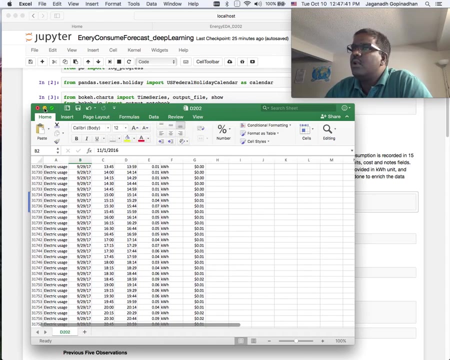 to 9: 30 2007. the data is available there. that means until september, uh, thirties of this month. the data is available there, there, from the pgand website. so i'm just going to um load this data um into a cwanta's data frame and start doing my data massage. 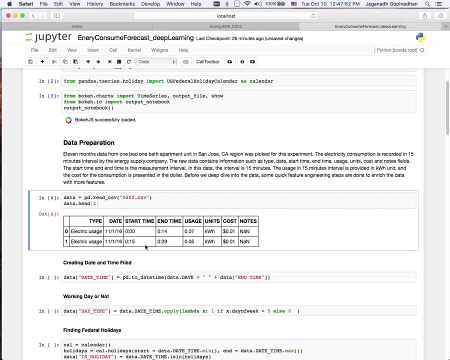 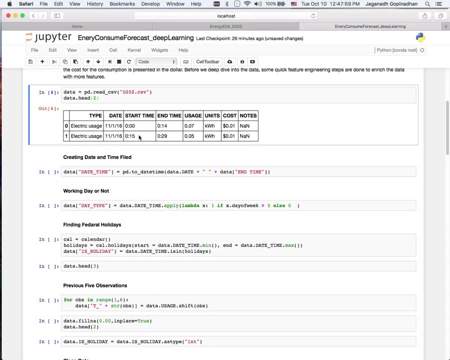 so just loading the data here- and i just taken to sample- you can see that the data- the head or the first two rows from the data- is exactly exactly same as we already seen in the in the excel file. so you can see that we have a date field here, a start time field here and the end time. 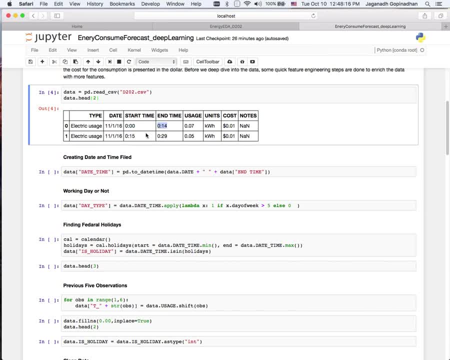 field here, but there's no such things like date and time combined available here. so, uh, what i'm trying to do is i'm trying to create a date and time field in this data up by concatenating the date and the end time. so why i'm taking the end time here? because 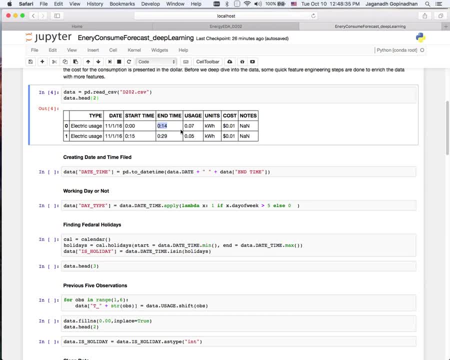 end time denotes when exactly the consumption is being recorded there. so that means when i concatenate 11: 1, 16, 0.014. so that means in the 14th minute of midnight i use 0.07 kilowatts. okay, i just wanted the exact time when this usage is being measured there. 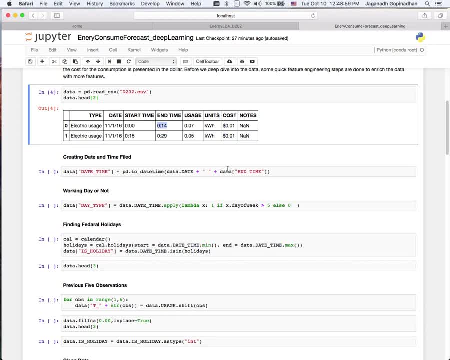 and from that time i can uh basically extract a bunch of new features uh in my data set to make my prediction more easy than the conventional autoregressive moving away or any other more such of such kind of like time series forecasting technique. so rather than just 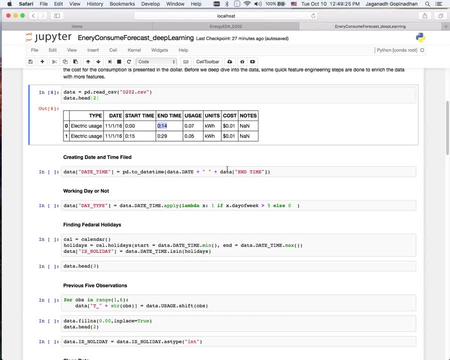 approaching this as a like conventional uh, time series forecasting. i'm putting that as a multi-varied time series forecasting here. so in that way, um, we are trying to like look at, look at the time series forecasting in the new dimension here. so so what we see in in the case of like 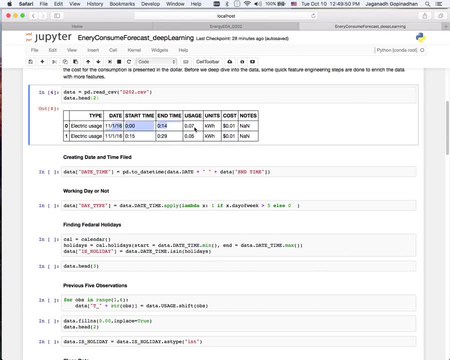 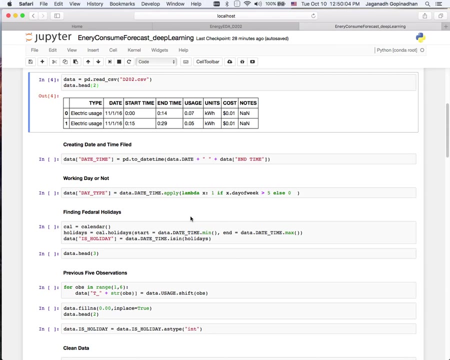 arima or any such model. we need this time and the consumption only, but from the data of what i'm trying to achieve here is trying to construct more and more features so that, so that i can, i can make more robust model by accommodating different factors or different other environmental attributes which is contributing to the energy consumption on a 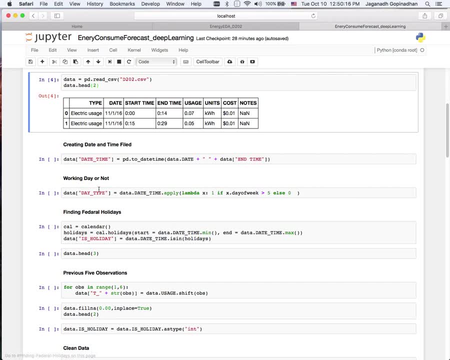 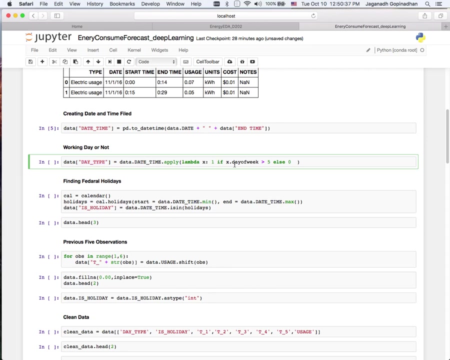 given 15 minute time frame, okay, so, after i have created this uh date and time field, okay, um, now what i'm going to look is that i'm going to create a new uh field in in my data called day time. what does the data means? is that, whether a given day is a working day or a weekend, so 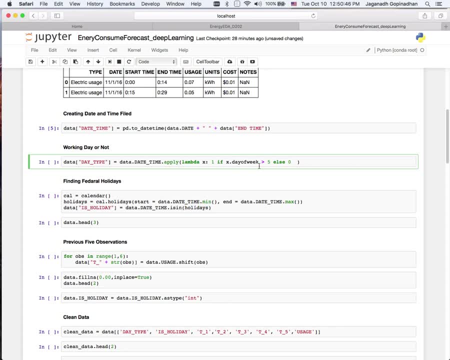 pandas: uh, the daytime data in pandas provides a convenient way to identify a working day. that means monday through friday. um, uh, we can identify, or any day we can identify easily from uh, from from a daytime object in pandas and then we can classify that in the working day or non-working. so what the logic? i'm? 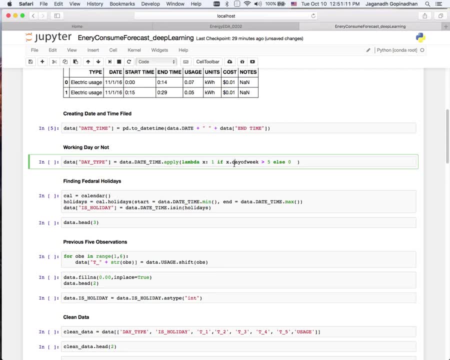 playing is that the day's starting uh to uh. from one to five, i'm categorizing it as a working day, and six and seven i'm putting it it aside- uh, non-working day. so if it's a working day, i'll I'll give the variable one, otherwise it's a zero. 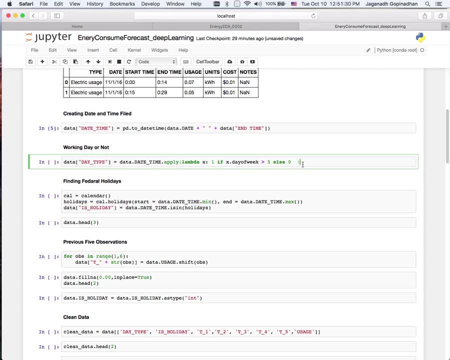 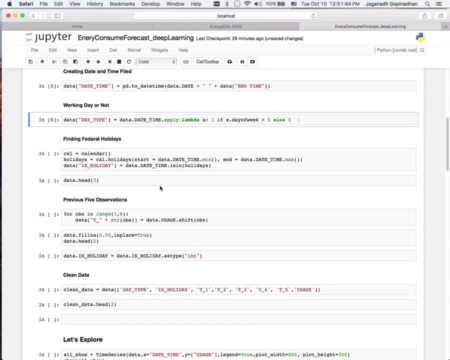 So it's a binary variable I'm creating there as a date time. So now, so we create the date time From the date time, I've created a new field called whether a given day is a working day or not. Now just wanted to understand out of the date time frame which we are like from November. 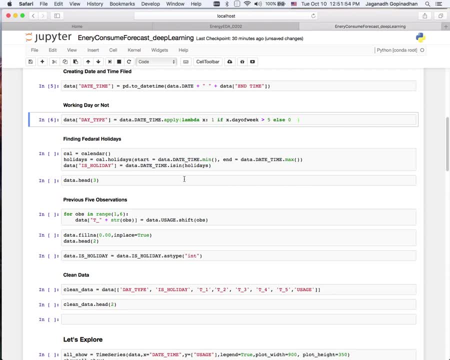 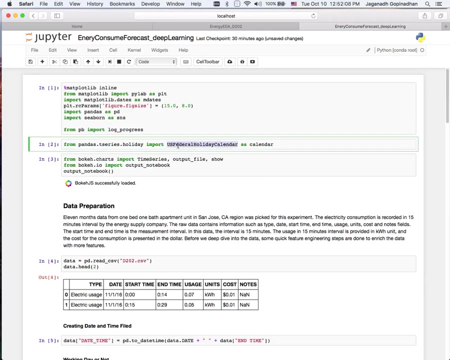 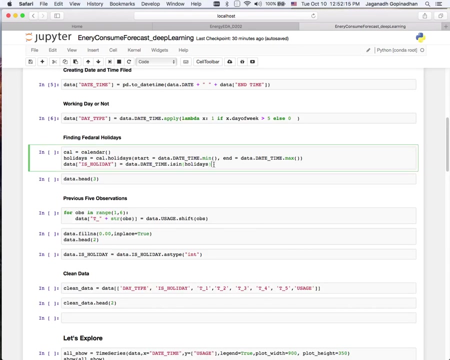 to September date frame in 16 to 17 period in the data set, just wanted to understand which of these days are federal holidays in this country. So, for the same, what I did is that I just imported my US federal holiday calendar attribute from the Pandas time series utilities and I'm just creating a calendar object from the 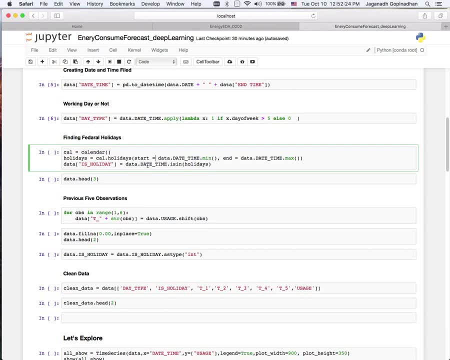 calendar. So the calendar object, what I'm saying is that get the holidays by the minimum date and maximum date. So in my data there is a minimum date that means the starting of November 1st and ending by September 30th of 2017.. 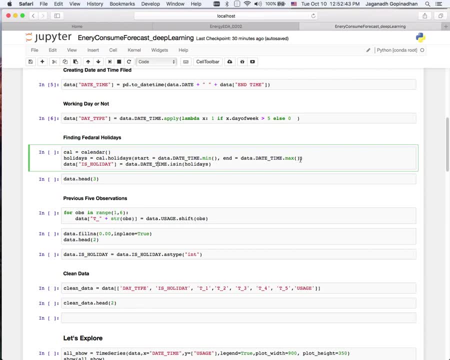 So find all the holidays which falls between these two date range, and then I'm just creating a variable called is holiday. So if any of this date falls in a holiday, there will be a true or false value will be applied in my data frame. 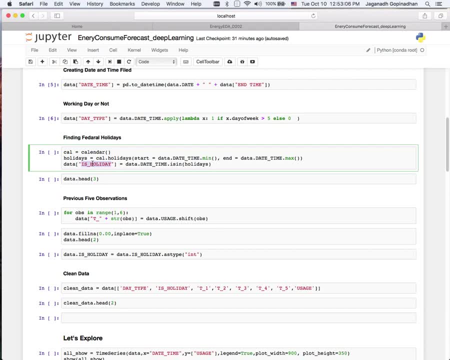 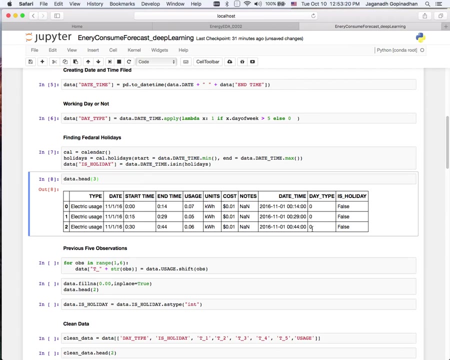 So an is holiday will be again. another, say binary variable which I'm creating with true or false values. So if you look into the data now, what we can see that I'm seeing like date type is zero. That means This is a, it's a holiday. 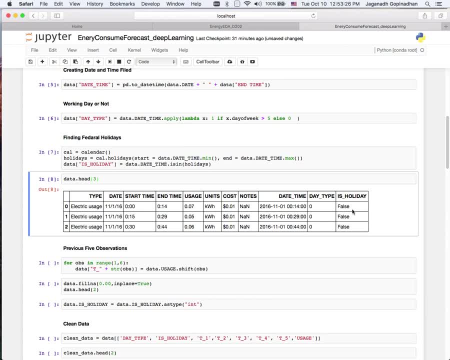 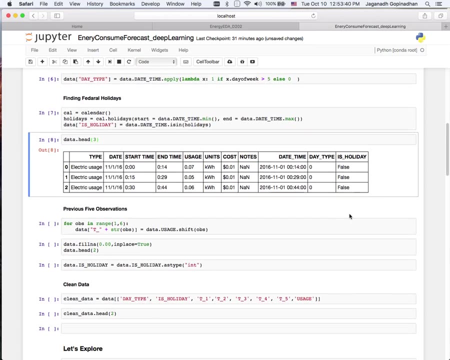 Okay, And and this holiday, whether this is a Saturday or Sunday, and each holiday means it's a, the particular day is not a, not coming under any of the federal holidays, such as Thanksgiving or Christmas, or any, any, any, any such day. 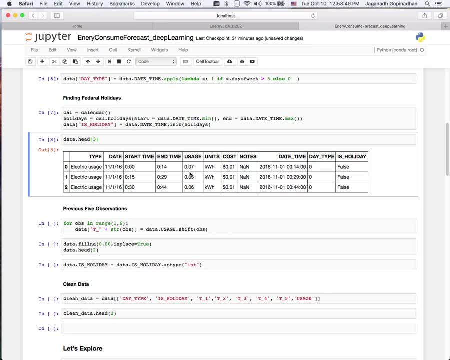 So from date and time. Now Let's look at some additional features or attribute in the data. The first data is the type of day, which says that, whether the day is a working day or a weekend, What is the significance of working day or non-working day in such kind of energy consumption? 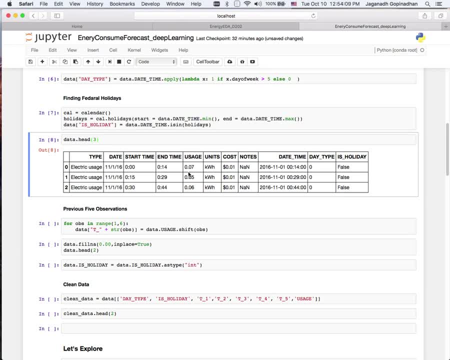 data is that if it is a working day, the number of people present in a household will be almost nearly half, or maybe zero, depending upon the occupant- occupants information. Okay, So that plays a very critical role in the energy consumption. Assume that it's a three member family, if three people are there at home and all the 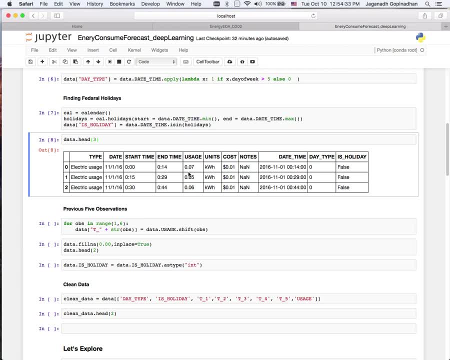 time, then obviously there will be more occupants working working there. So, for example, somebody may be charging their mobile phone and laptop is being operated, TV is being operated, Maybe it may be using a fan or AC. more lights will be operated during the daytime. 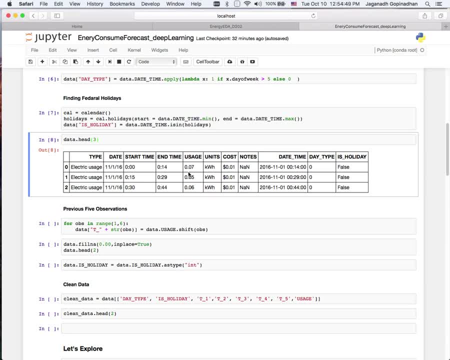 So you can see that a steady energy consumption going there. Okay, So since it's a weekend, so you may have some special cooking going on there. You may bake or boil something, So more electricity is being used in your kitchen also. So all these things basically affects there. 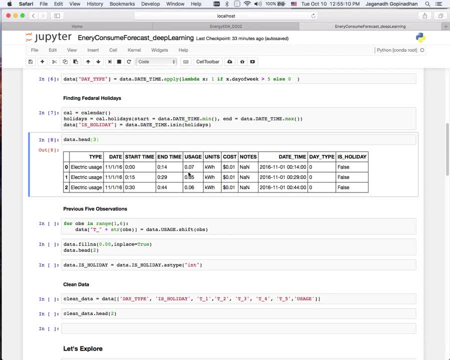 So that's, that's a specific significance of the data. So if the three member- and one is a student and one is working and one is non-working, that means during the daytime. So during the daytime the maximum population at home will be like only one person and that. 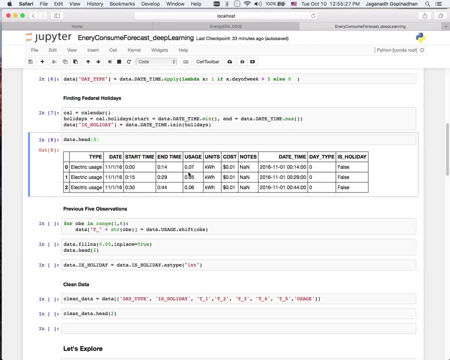 will be between the like, say, 830 to six, between 830 to 6pm, 830 and the 6, 6pm. So during that time again the number of uh, electric, uh or electricity consuming gadgets use will be very less. maybe a TV, a laptop, occasional charging of a mobile. 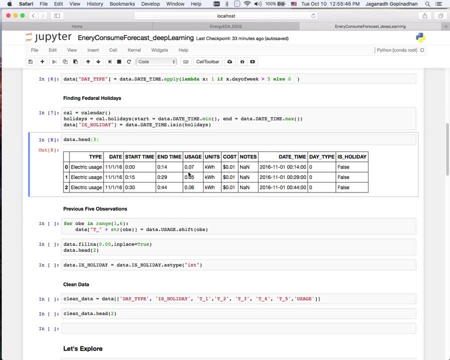 phone, then occasional cooking. Yeah, So at the moment, after 6pm, all the three members are at home. Suddenly somebody brews coffee, tea, opens the fridge. the consumption starts up there, Right? That's the significance of the type of day. 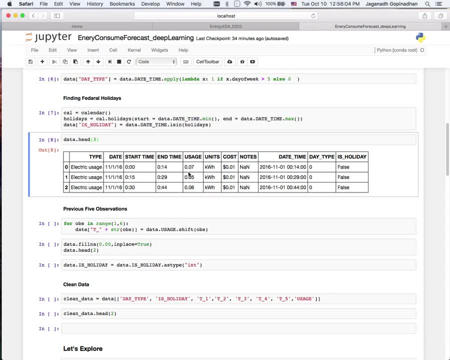 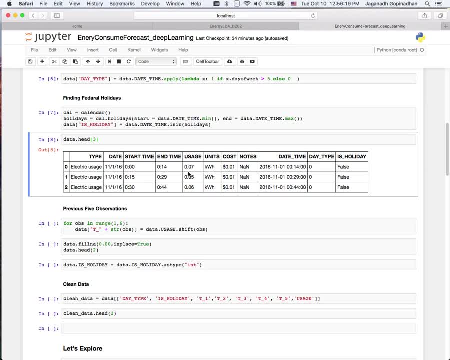 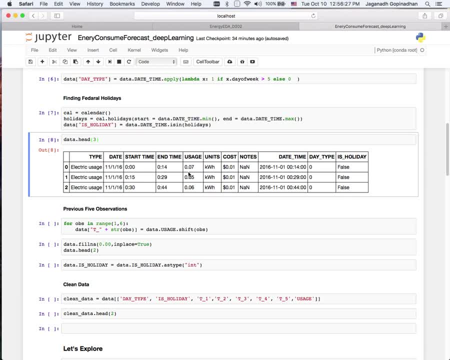 or something. So it all adds up consuming additional electricity in in the kitchen area. So these two variables say that, whether our increased conception has something to do with a particular uh day type or a holiday, So I'm just stopping uh creating. 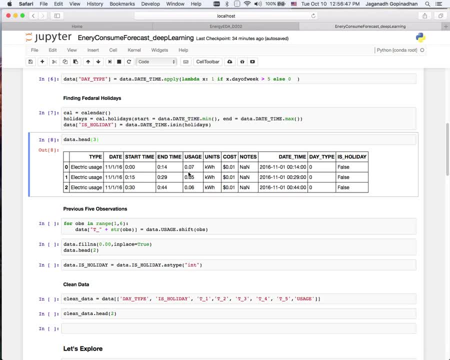 Some of the details. Okay, Okay, Okay, Okay, Okay, Okay, Okay, such time related feature here. you can be more creative in this area and you can try to create some more extra variables, such as you can divide the day into different parts, such as early morning. 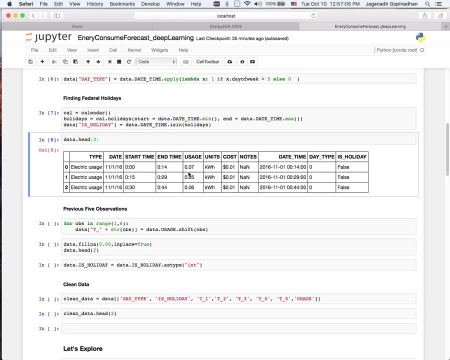 morning that day and evening and night time. so what it signifies, such kind of a variable is like typical. in a typical household, the day may start by 6 am. everybody wakes up. you brew your coffee, tea, your breakfast cooking, the lunch cooking, everything happens. maybe all these? 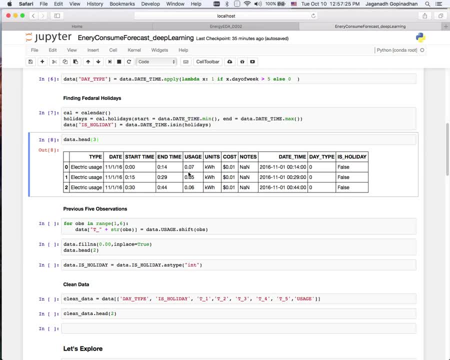 things may come to an end almost by say like 8, 39 a time, and this time it will be a busy consumption time or it may be referred as a peak time. consumption, uh, consumption, uh, consumption for the electric equipment. and then, nine o'clock, like people go for their own daily routines, go to. 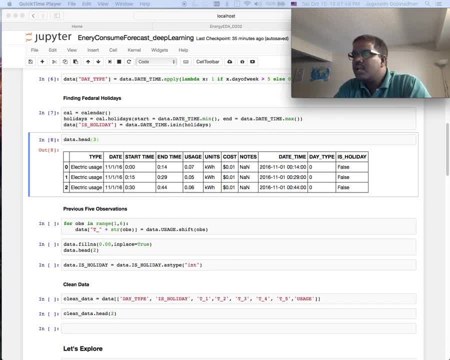 school, college, etc. so now the routine equipments may be only functioning there. so, and in the evening you come back again, you brew tea, coffee, make dinner, and then all these things again starts consuming more and more power. so now we can see that dividing the day into multiple 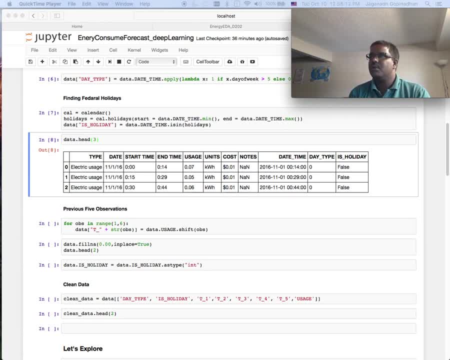 parts is adding additional information about your data. what affects the consumption there is. you can even bring some external data which your energy construction company or the energy company may not bring, such as the weather data. you can go to the noaa website and now download more detail about your region and what was the temperature, etc. so why does temperature, wind, rain? 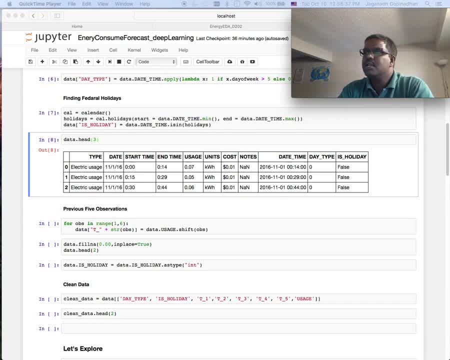 or any such attributes affect the energy consumption. because if the outside temperature is 10 degrees centigrade it is very obvious that you put um the room heater on. that consumes more energy. obviously, if the outside temperature is 35 degrees centigrade, you put your ac on, you may put fan or you may connect more portable uh coolers there. 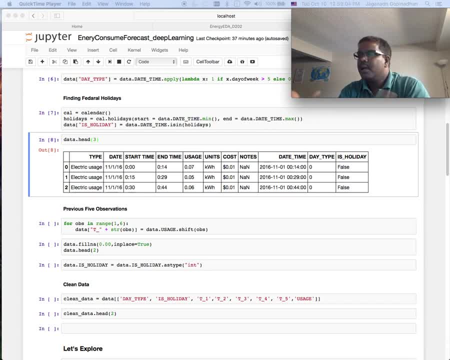 so it again starts, uh, increasing the um and increasing the energy consumption in your household. so, apart from the features which we just constructed here, you can construct more features, such as the weather information or any such informal which you can create up from external sources which may have a significant influence, uh, in your electricity. 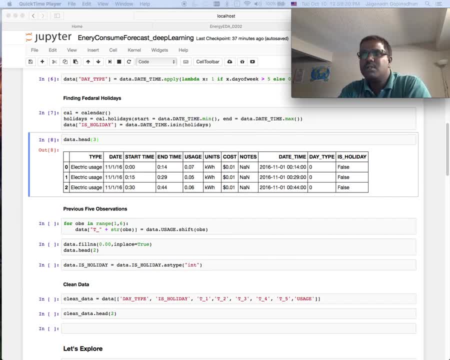 consumption can also be used here. but in the part of this tutorial i'm not trying to bring all such additional data or anything, but you can try it from your end and see how well you can make the forecast- yeah, forecast, uh, forecast- in in future. so it's, it's one of the creative way of doing more and bringing more and more feature, or 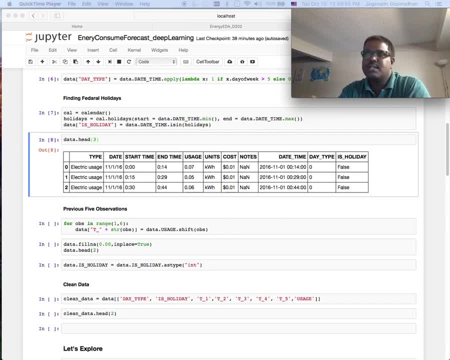 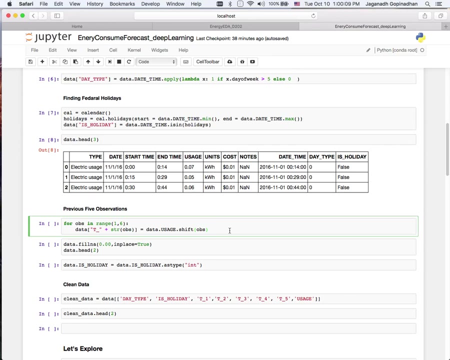 doing the so-called feature engineering, feature addition, etc. to make your forecast more and more accurate. so now, uh, after this, what i'm trying to do is i'm trying to create some more additional variable, say. basically, i'm trying to, um, trying to create, uh, five new, uh, additional additional fields. 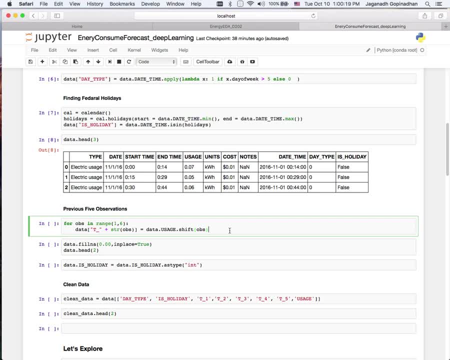 of data. that is nothing but copying the the previous five energy consumption details. uh details say i mean yeah, i mean in the time of like 14th minute of the day, that means um 12, 14.. so what i do is that i'm just trying to copy uh 5, 15 minutes information there. so pandas. 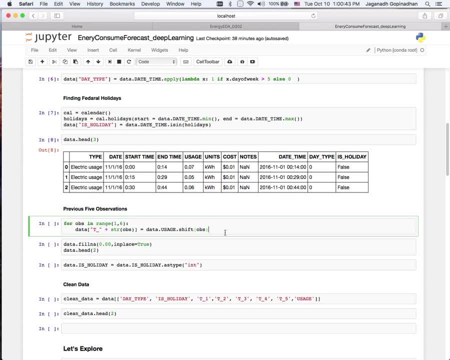 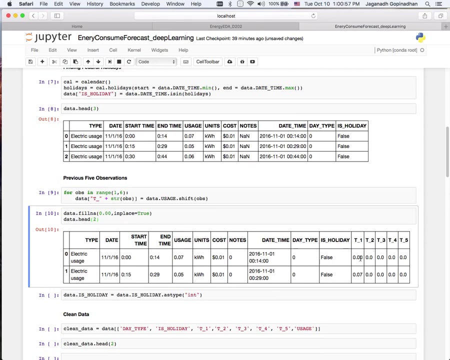 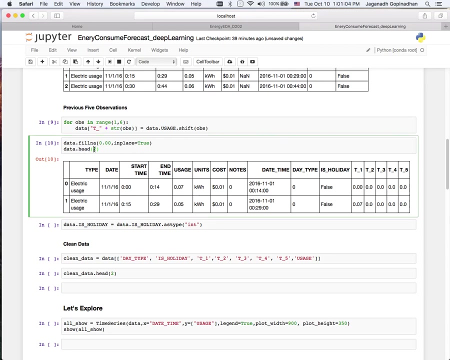 gives a very, very basic utility. to do that, uh, using the shift function, just doing that magic here and somewhere, you will be having some zeros coming there. so i'm just just filling those zeros and i just created, um, five additional additional attributes, the data, such as t1, t2, t3, t4 and t5, which is basically so, like um, uh, copying information from the previous. 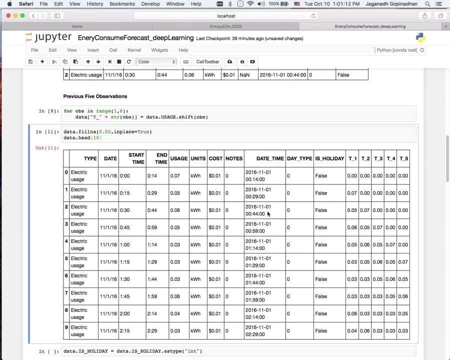 file. so i'm just taking the top 10 information. you can see that say in this one. so you can see that the t1 information you are seeing that i'm copying the usage from here to here and this information is coming here. this information is coming here so you can see that the information is flowing from. 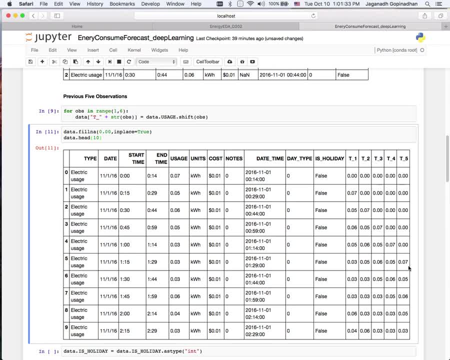 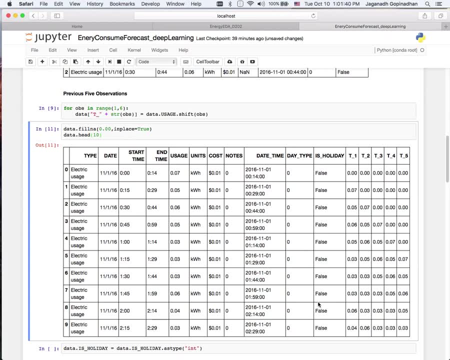 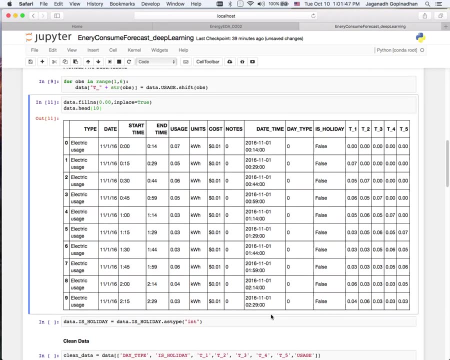 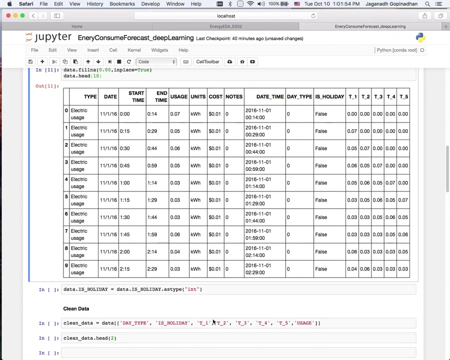 here to here to here to here. here i'm copying the previous observation here um such as a reference to how much i i consume in the past. so that also sometimes affect how much i was consuming earlier also affects how much i may consume next sometimes. so i'm just creating that, that attribute here in. 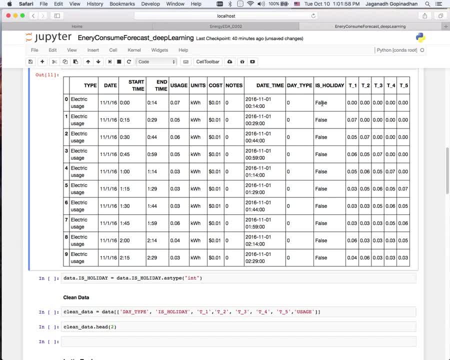 in in in my data. so if you look here, this holiday is now appearing as a like, a true or false or a string variable kind of thing. i'm just trying to convert that in the in the into the basically um integer type, so that it will be now appear as: 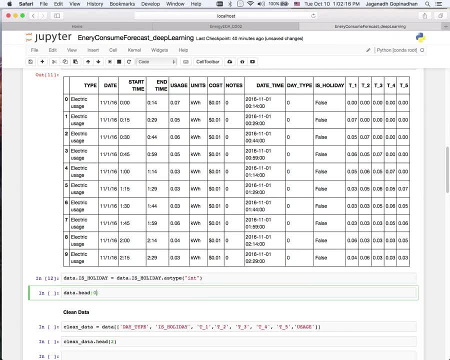 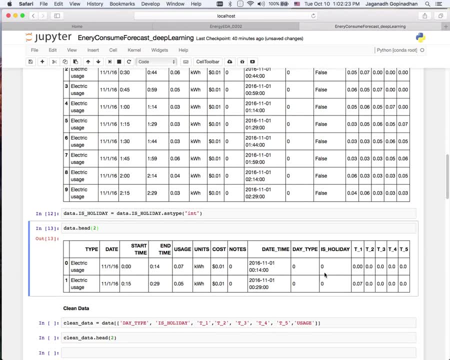 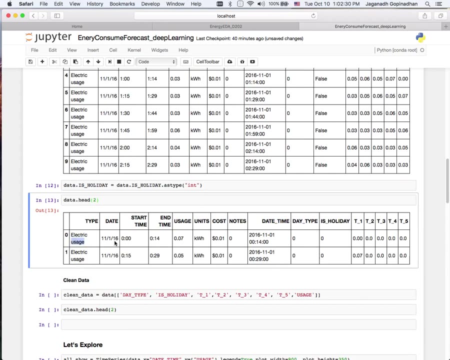 as 0 or 1, and now we can see that these holidays now appeared at 0 or 1, kind of a variable here. So if you look here, I don't need the type information, the date, the start time, the end. 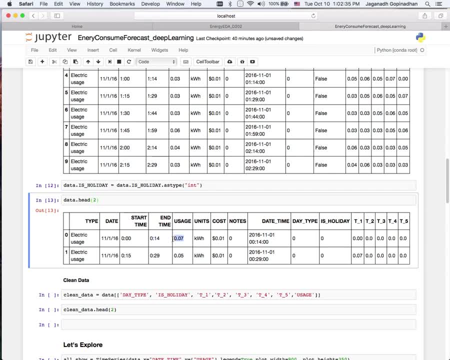 time. Obviously I need the usage because that is what my target is or that is what I'm going to predict. The kilowatt hour, the unit information is not required, Cost- I'm not going to use in my forecast, Nodes is not required and obviously the date time I'm not required right now for forecasting. 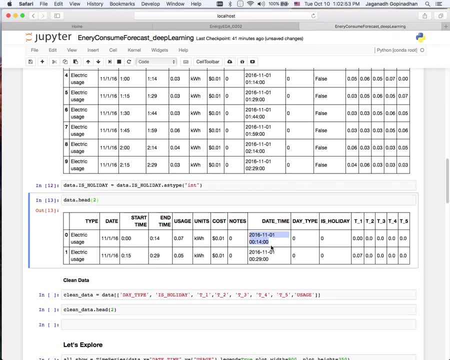 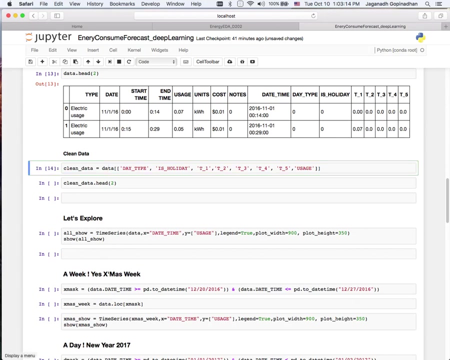 because I already decomposed the nodes field and now have something which is better than the date time field here, and date type is holiday, t1 to t5.. These are going to be my primary information for creating nodes. So just demonstrating here how I'm just creating a cleaned data set or a data set which was only 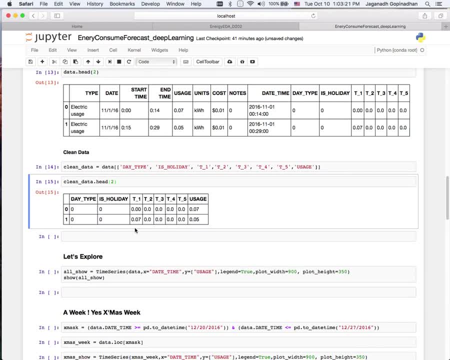 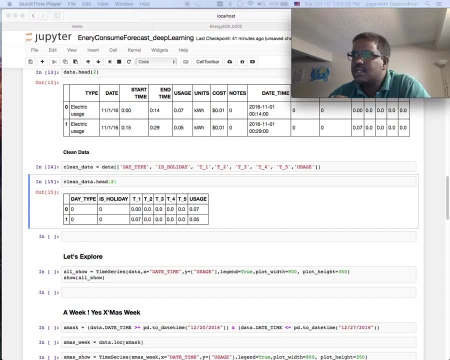 the required information for building the model. So this is so far. what we did is that we just created a bunch of additional attributes and also I was just telling about how can we create more attributes. So now let's try to see, or we can have a closer look on what is there in the data. 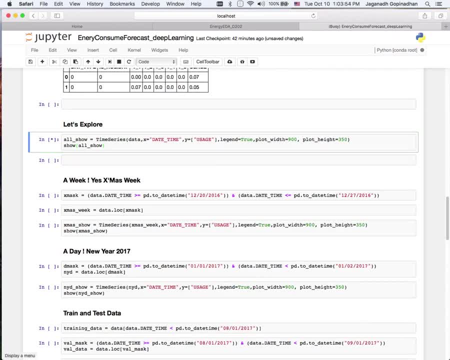 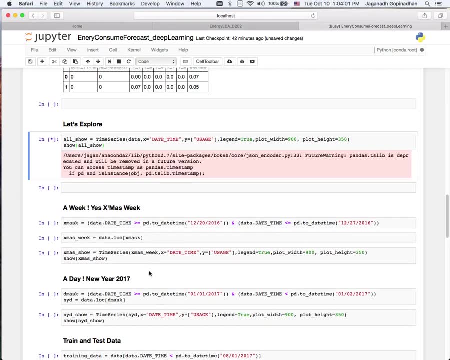 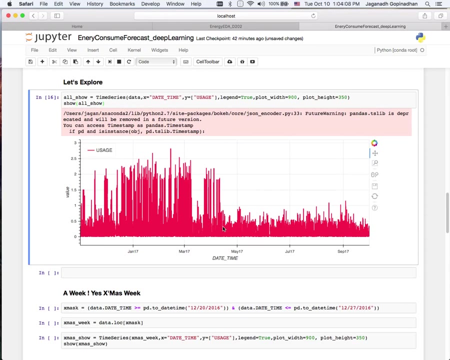 So I'm just using the bokeh library from anaconda to create an interactive plot of the entire data. So you can see that it's now giving you a plot of the entire data, of the of the, say, like the 10 months data is being plotted here. So I can, I can just zoom and show you. 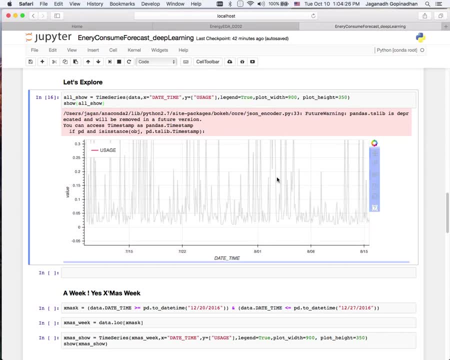 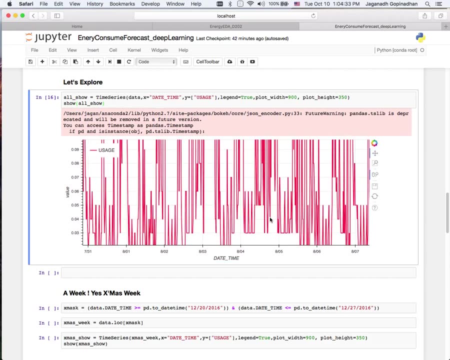 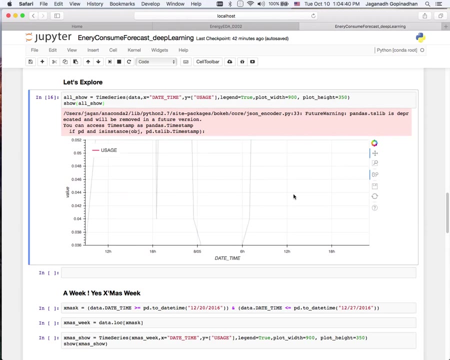 some of the information I can zoom and show you. Yeah, so there's a beauty of using a bokeh library. So it has an option to like, pan and zoom the data in a much, much, much better way. So you can see that. so it's too much. 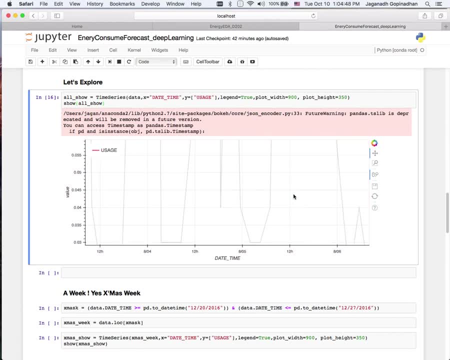 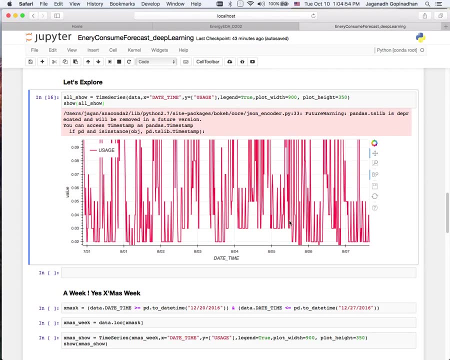 You can have a close look on the data by zooming here. otherwise your slice undies the data again and again if we use a libraries like ggplot or, or, or this or country plot clip kind of the library here, Sorry, So you can see the. 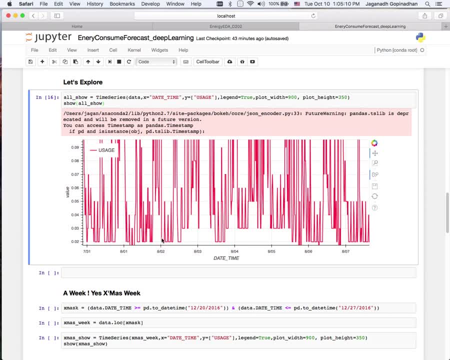 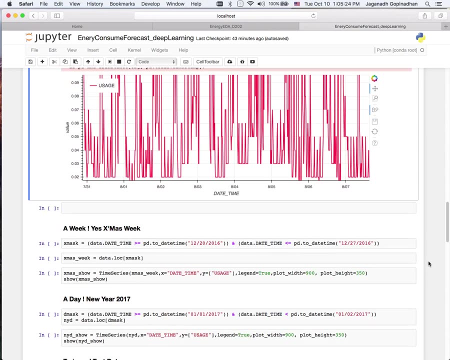 So there's lots of peaks and valleys in this data. basically, that signifies that the peak signifies that whenever I'm using more electricity, while I'm using electricity in a very steady manner, that I'm running some of the routine electric appliance, such as fridge or some decorative lights, etc. 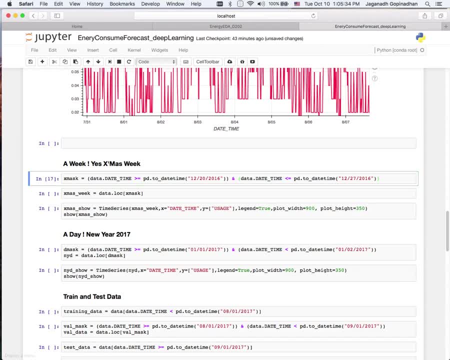 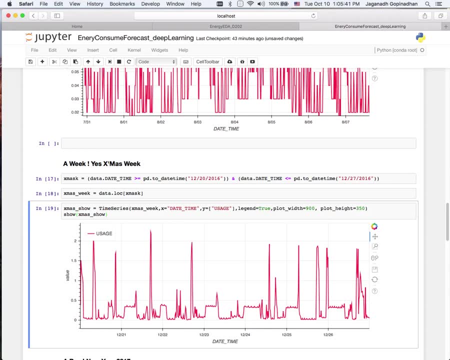 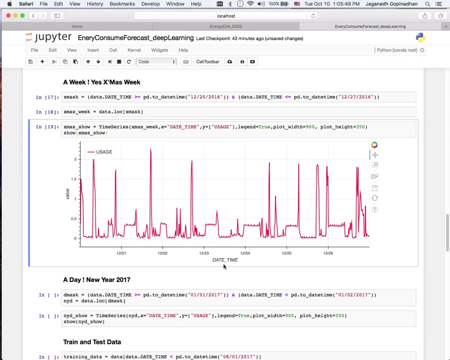 So let's take a more closer look on the data. I'm just trying to extract only the data from the Christmas week. You can see that the Christmas week means I'm just starting from December 20th to 26th to 27th to midnight in my data. 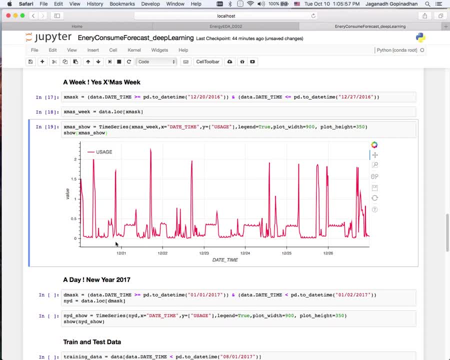 You can. you can see that. yeah, there are certain peaks, always visible in early morning and evening, morning and evening. the peaks are mostly appearing in the morning, evening and evening. So yeah, I'm just trying to extract only the data from the Christmas week. 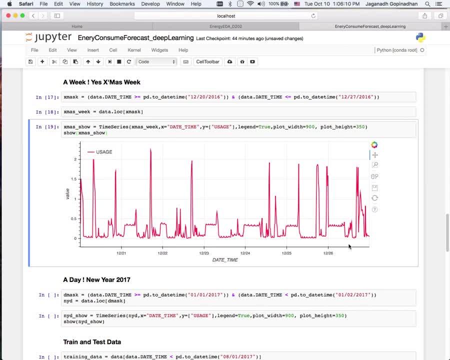 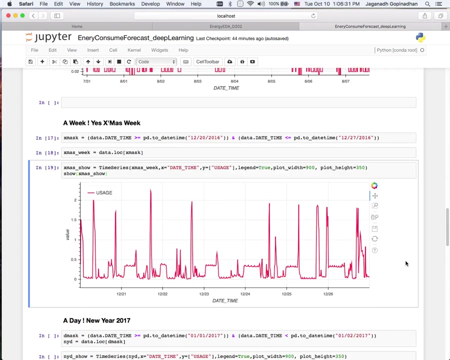 evening and there is almost a steady consumption throughout the day and in the night you can see some sort of spikes appearing here because it's a really cold weather. so we may need a room heater to heat up our home so that we can stay warm inside, kind of thing. 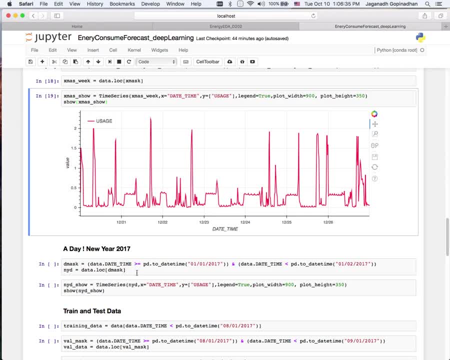 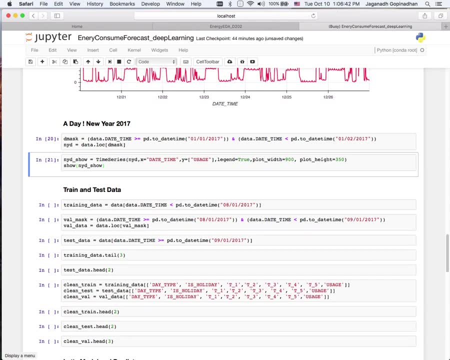 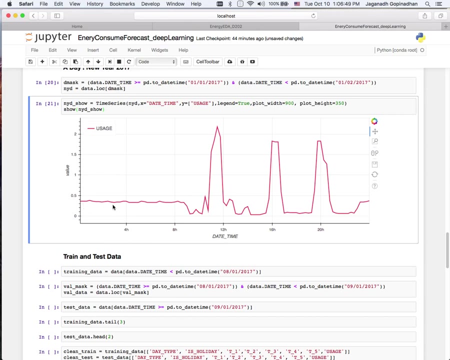 So that is what the data more closer look of the data reveals there. So let's zoom down to a single day. So I'm just going to the New Year day at 2017.. You can see that throughout the night, we were having like or consuming about 0.4 kilowatts. 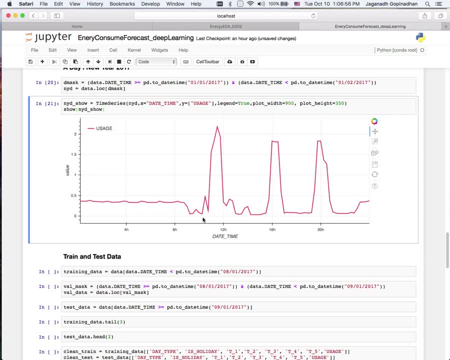 per hour and till say, like something like 8.39, and so on. we switched to our room heater and started making tea, coffee, lunch, dinner and so on. So as we have the heat of the summer, everything starts, the consumption goes into its peak. 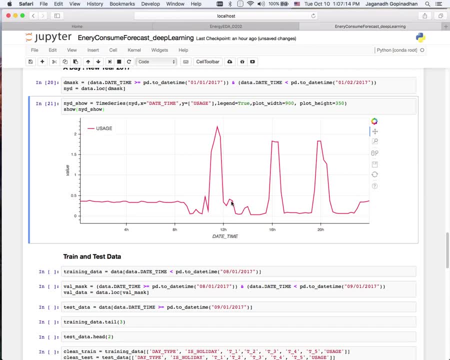 And now we are taking rest after our grand New Year lunch. It's going to be the evening, the dinner time and at the evening time, so the tea, coffee to keep us warm. everything is being prepared here at the 4 PM. 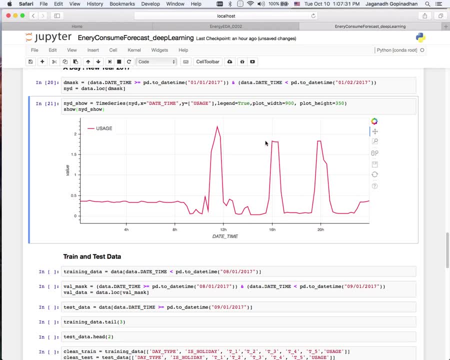 We can have a steady electricity consumption peak, appearing here in the fourth hour and again straight coming back to the summer. So it's going to be a pretty good day: life, warming our dinner, and then we are going to fire up our own heater. that's where it's. 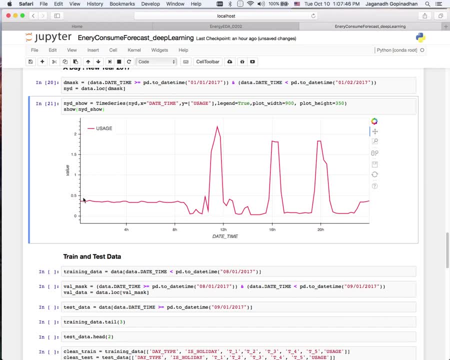 going, you see. so in the zoom data of a single day, you can see all the story. you can narrate all the stages, all the story of what your family is doing throughout the day. if you know, if you know it in a better manner, that's what the data clearly signify. so that is what 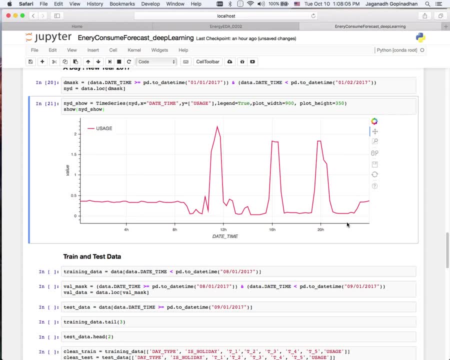 I was talking earlier. so the better if you can construct more time-related features from your data, the better it is trying to explain you how good, or how the or what affects why the consumption is going up and down in your apartment building. so those features, some of those features we already constructed from our data, some are just given us a feature. 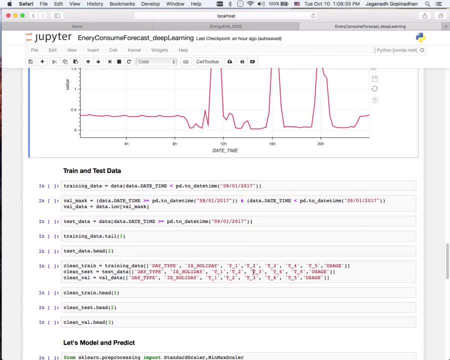 so now what I'm going to do is that us you're going to start our data science model building. so you know that, as a standard practice, we need to create train validation and testing data. so what I'm going to do is that I'm going to keep all the data till 7th month of 2017. 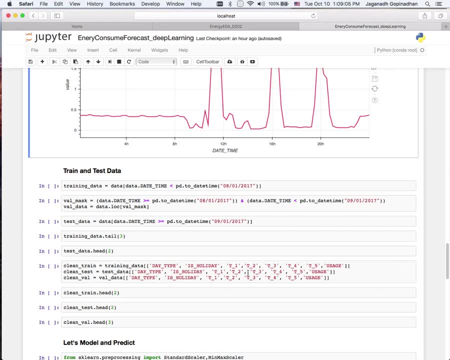 okay as my training data, which comes around 8 months worth of data as my training data and I'm just trying to keep one month data as my validation data and I'm just taking two month worth of data as my final testing data for the for the model. 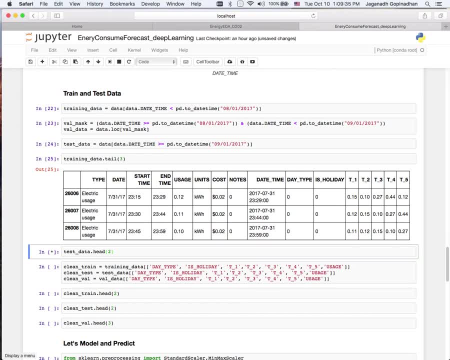 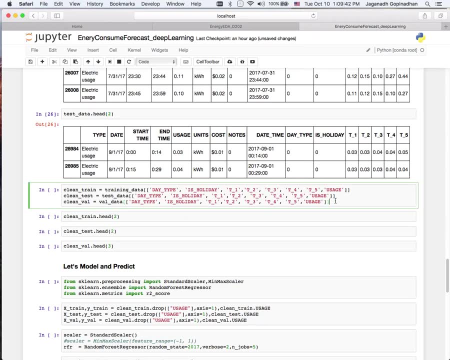 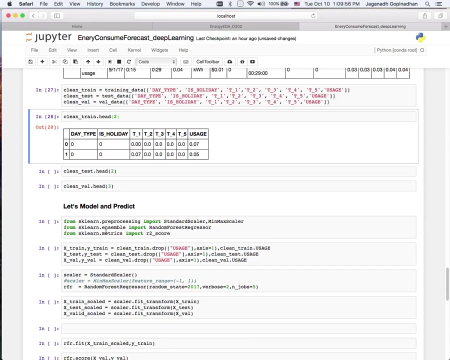 This is what I look of for the slice of data which which we created here. okay, and and from the data. so what I do is I just just pull out the required information, such as day time, holiday time, 12 time, 5 and the target variable usage here. so I just pull out those information from the training test and validation so you can see the the train data. 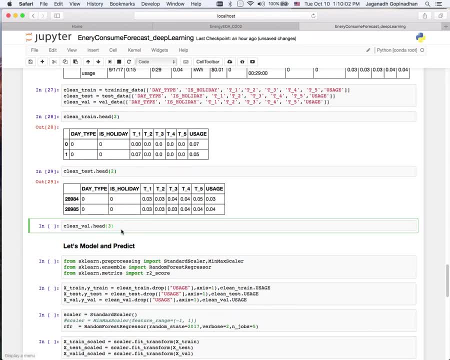 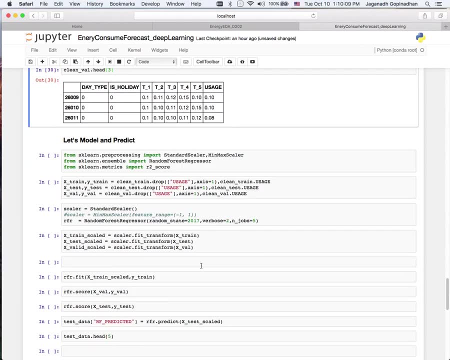 train data and and the test data and the validation data, how it looks okay. so to start with, I need a very, very baseline model. so what I'm going to do here is like I'm building a very minimal, random forest regression model as my baseline model. just listen that in the case of 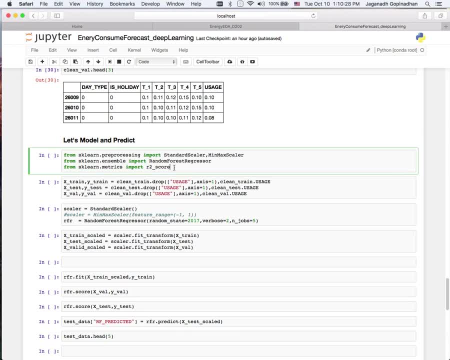 reference to see how the model works etc. so I'm just importing the scale in random forest libraries here and and the min-max color folder, like basically to scale my data extra and here in this box what I'm trying to do is that I'm just creating my train X and Y variable for my training. that means that means my 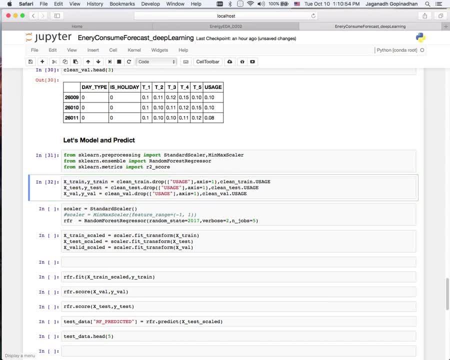 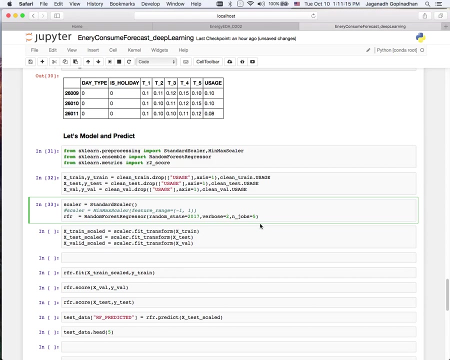 dependent independent variables. I mean extracting from the data, from training, test and validation data, and I create the object of my scalar, standard scalar or the data scalar function and the random forest regressor. I'm not doing much of a parameter tuning here in my random forest regressor as I just just use the default values there. so bet me it's not going to. 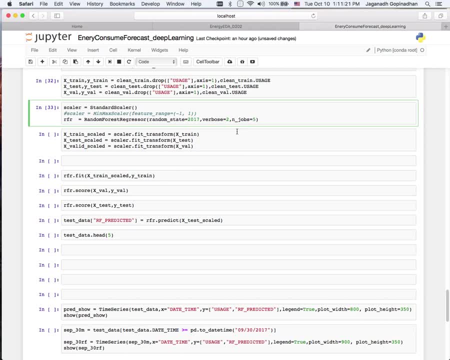 be a very, very robust model. I know, since I'm not tuning the, tuning the tree, or I'm not going to like fine-tune the depth of the tree, etc. nothing, it's all, all a very basic task specified in the scale and maybe I'm going to use it here and the 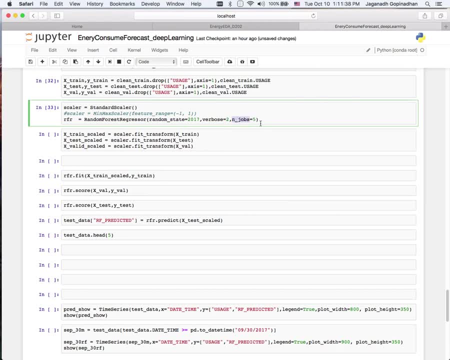 only thing which I'm going to use is an end job is equal to five. that means it's a parallel a to around five jobs to five parallel jobs in to build a model that basically makes the model building little bit faster. that's it, so that's. 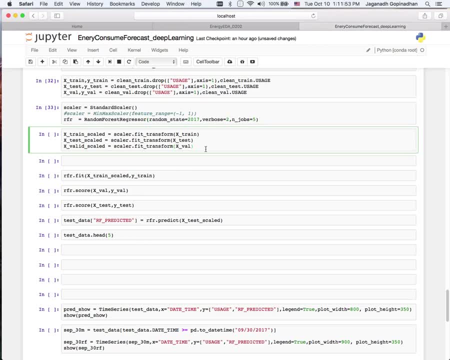 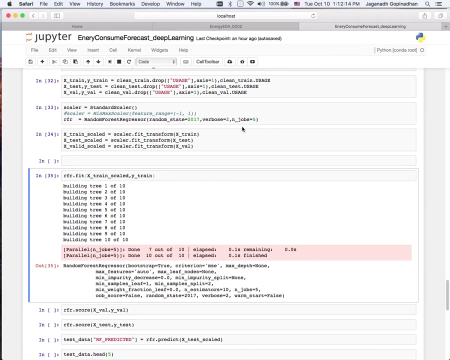 not a hyperparameter, that's basically an execution one. and now I'm just going to scale- scale all my data here with the standard scalar function, here and now. Tata, we are just trying to build the model. okay, since it's where it's a parallel to one number of jobs, five and 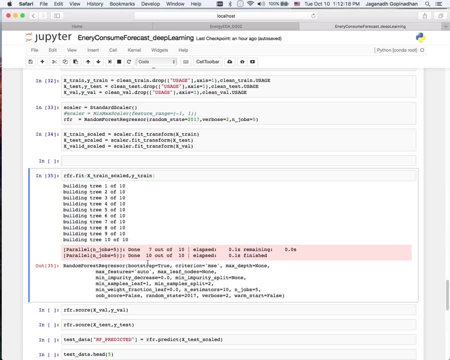 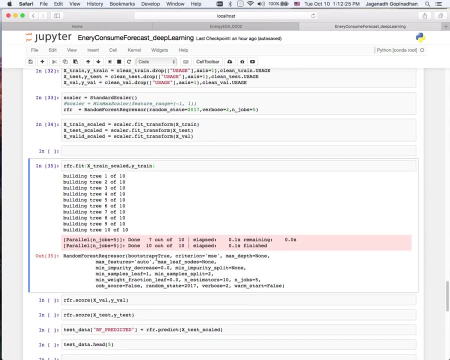 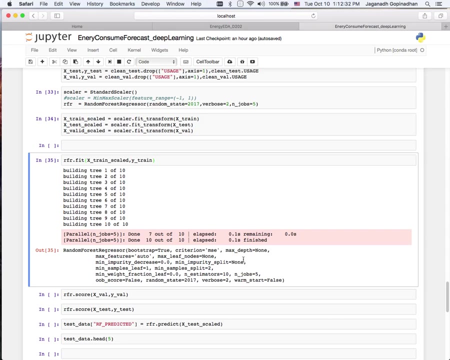 I'm having a like quad core machine, so build the model in a fraction of a second. you can see that. what are the hyperparameters here from this output? so I'm using the bootstrap. it must be of the criteria and maximum depth I never specified for the tree, the 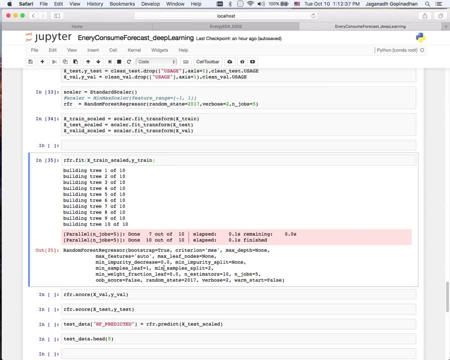 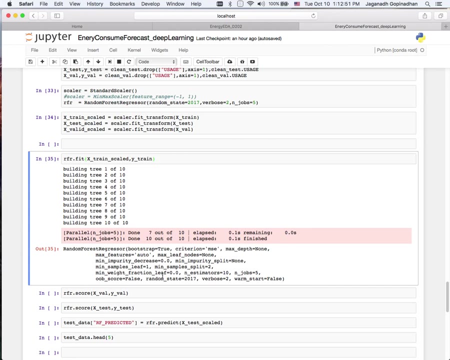 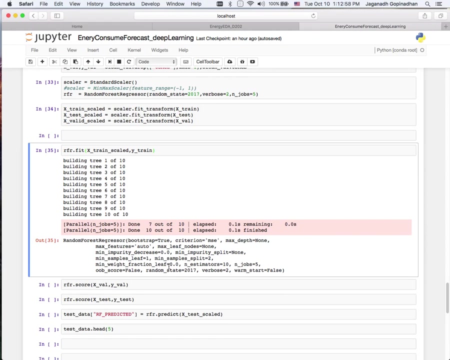 maximum features. it is determined with auto algorithms there. the impurity decrease and minimum purity split etc. are very, very normal as specified in the library- and I'm not using all these scoring or nothing, okay. so even the warm starting is also not specified there. so the default parameter settings are being 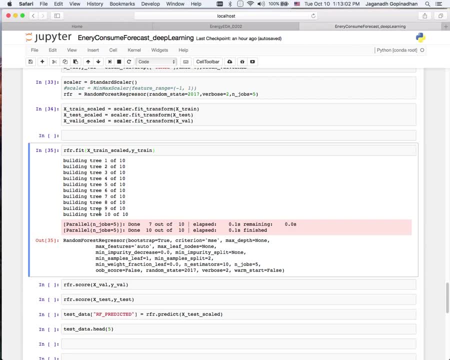 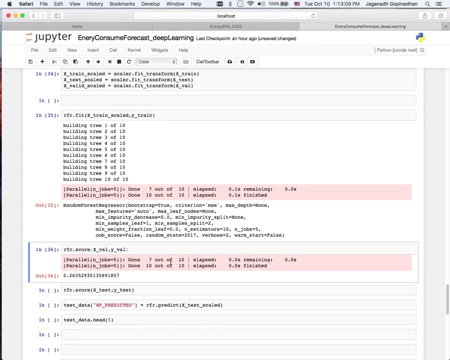 used, except in the case of number of jobs, and they just will take very basic model here. so let's see what is the R square value in my validation data. so the R square value is 0.26. that means it's able to explain only 26% of the 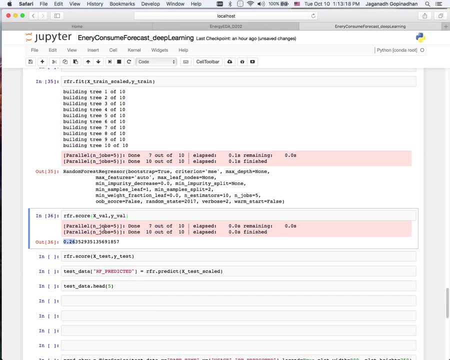 variance in the data database. it from my model. so, yeah, that means that all the model is not so good. and let's see how much is the what it was a R square value in my test data. so I'm just building a very basic model and I'm not using all the 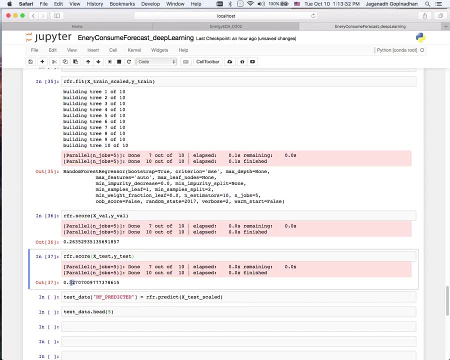 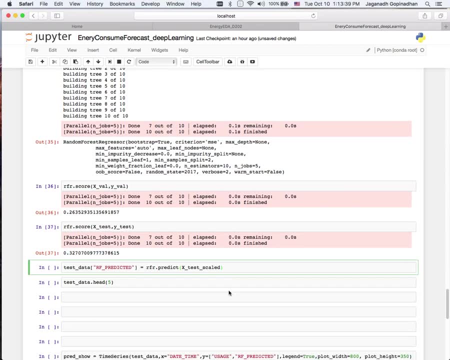 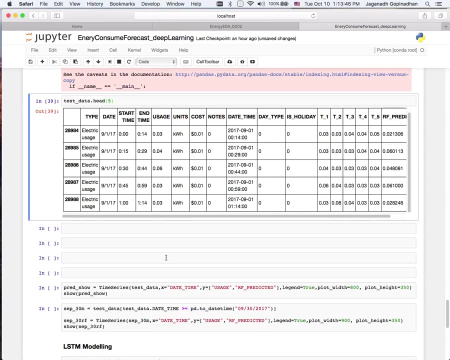 data and the test data also having the r square of 0.32, that means 32 percent of the variance- is being explained here, um. so let's try to like basically visualize, um, visualize the result. to visualize the result, what i do is that i just added the random forest predictor result. 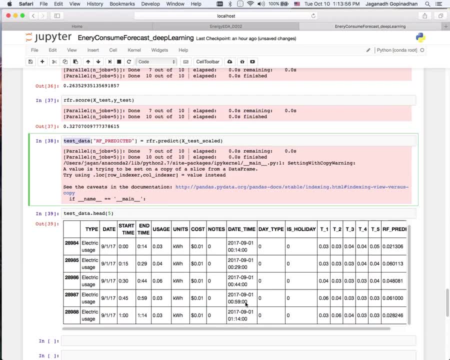 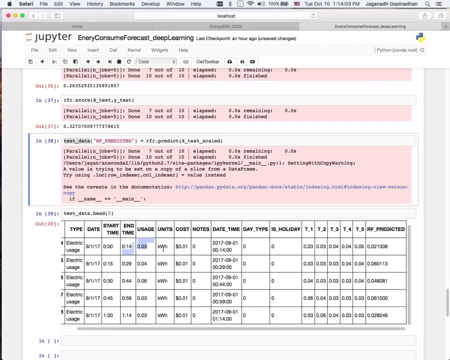 to my test data data frame, fundus data frame and this is how it looks. my predictions will be here. you see that the usage of 0.03, i predict rate as 0.02. here they say 0.04, i predict rate of 0.06. 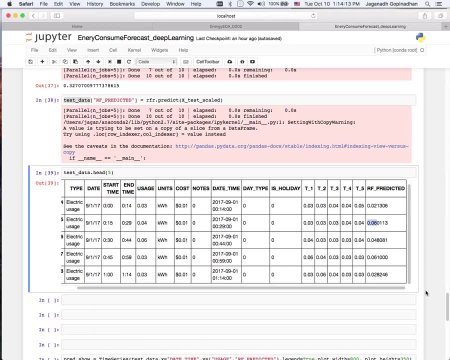 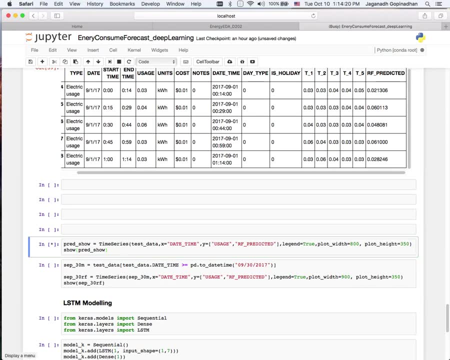 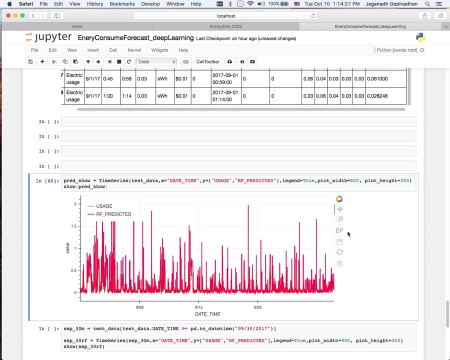 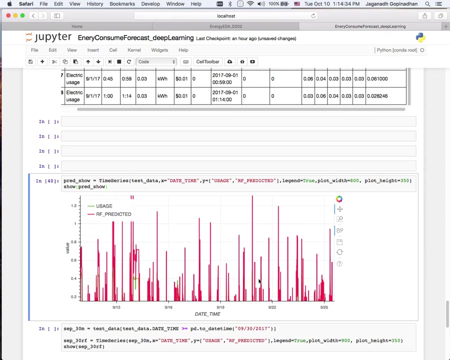 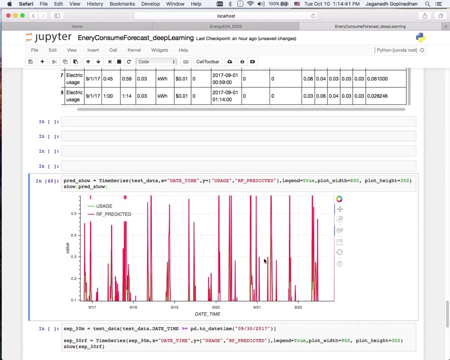 so you can see that, yeah, some obvious, um, obvious, additional predictions. i did, okay, let's see by how good our prediction is. okay, so you can see that, uh, from this data. so you can, you can. so let me zoom in. they're almost there, kind of almost very close, but not so close. that's what i say. 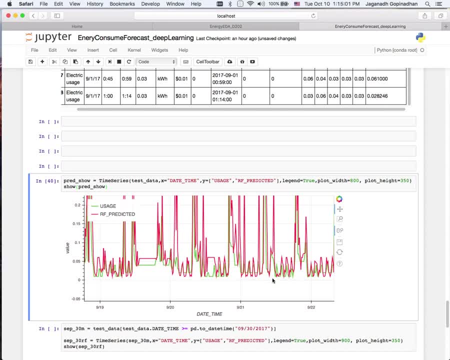 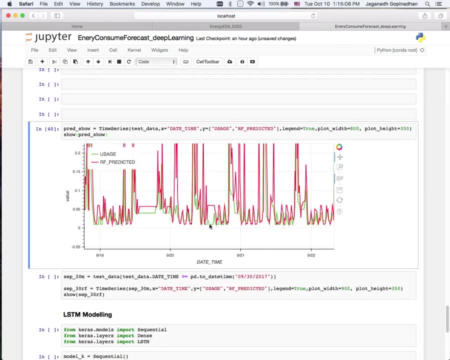 it's not so robust. yeah, some of the peaks and valleys we are trying to replicate, but not very close to those peaks and valleys. okay, and here you can clearly see that this is my actual usage: i'm predicting way too high than that. see, look, here i'll turn predicting way too high than 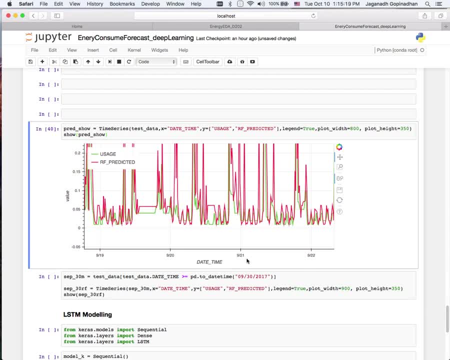 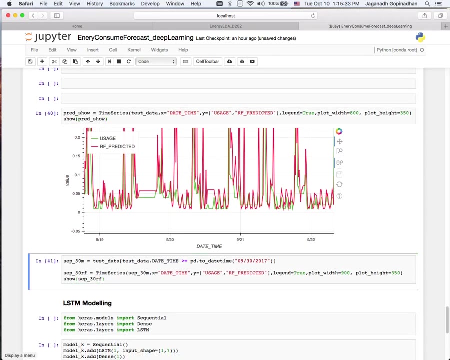 what actually was consuming there. so that means the model is not performing well where it required. but if you look here- some of the peaks- it was able to clearly make a matching predictions here. so let's make a very close look. so how much electricity i was consuming in september 13 and how much 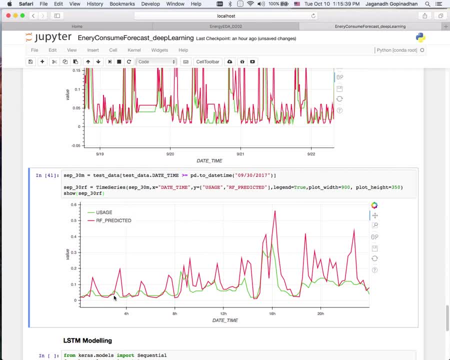 that is on september, and how much i'm predicting. oh see, here you can see that in the midnight it is saying that i may use almost 1.5 kilowatts, but my actual consumption was 0.5 kilowatts kind of thing. but between 8 am to 11 am the prediction. 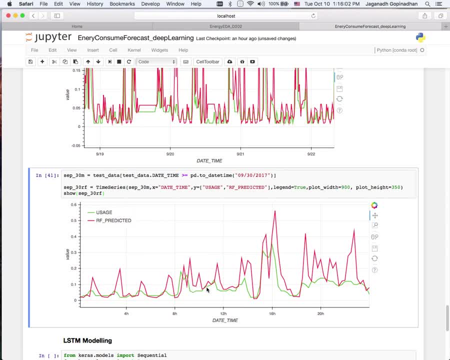 matches, but not exactly, because the peaks are predicted in a different way. maybe it might have indirectly guessed that i might have wake up by 8, 45 or something, maybe okay after 12. so it's saying that like okay, this, this part is, the predictions are way too high. so yeah, well from. 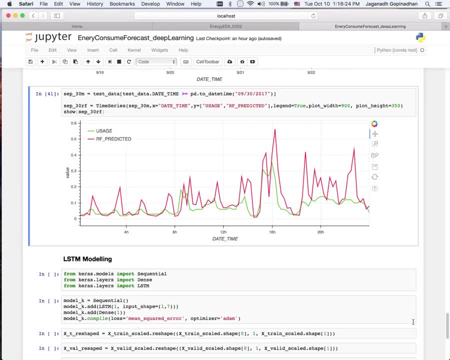 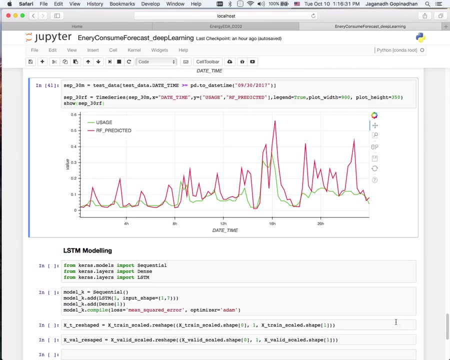 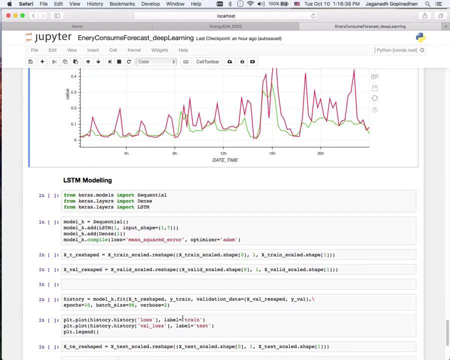 the r square value and from the plots it's very obvious that, okay, the predictions are not going to be good. but, as i promised, this is not deep planning. we just do the typical ensemble or or a tree based model. here that's a random forest one. so our objective is to build a build a deep. 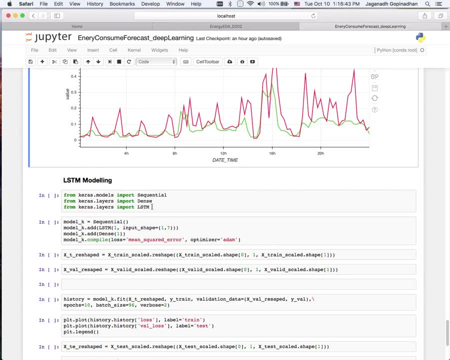 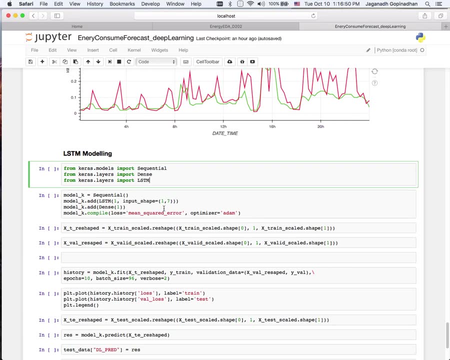 learning model. so here, what i'm trying to build is a, is an lstm model. so lstm means long short time memory network, which is uh proposed in 1997, uh as a, as a neural network enhancement and uh by the uh uh advent of all these new deep learning frameworks, libraries and gpus, if you. tpu review. 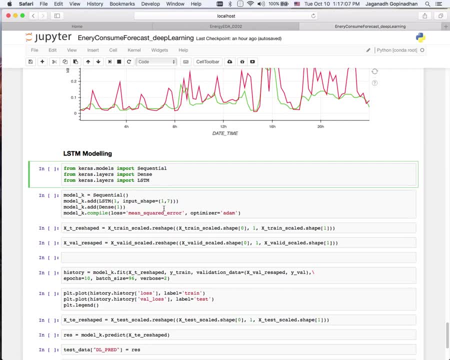 kind of all this revolution. this kind of algorithm becomes very popular, apart from the convolution neural network which we use for uh image, uh image image based machine learning or data science, or a models for natural language processing, time series, forecasting or any kind of sequence. um sequencing problems in machine learning, we use lstm nowadays. 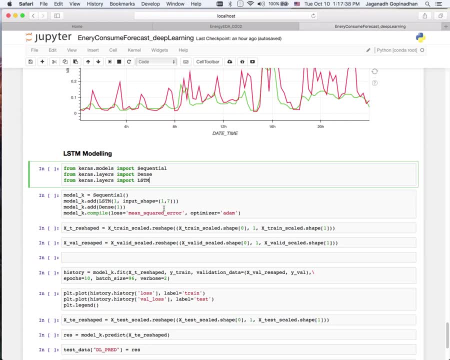 so this is a kind of an uh, considered as a kind of an enhancement to the, the recurrent neural network, which which always look back into the previous observation and tries to make the prediction. so you can have a deeper reading uh from andrej karpathy's tutorial. 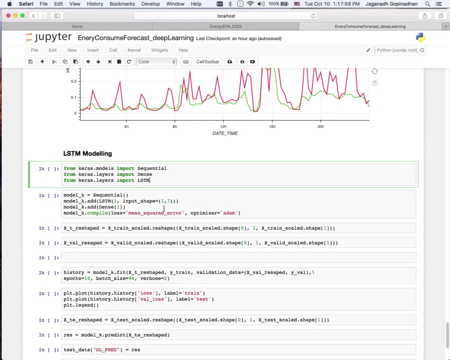 on on deep learning and you can try to understand what is rnn and what, what is lstm, and there are lots of online material available there. i may not be the right person to give a theoretical view on on that, so since it is already, the internet is already filled with, uh, tons and tons of material. on this day planning aspect, rather, i thought i 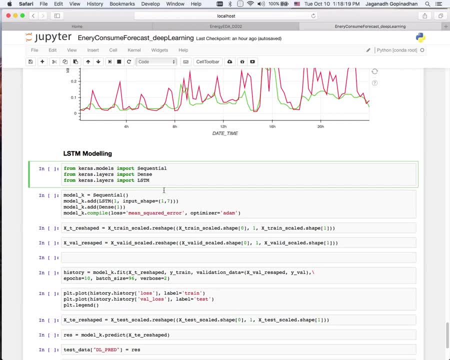 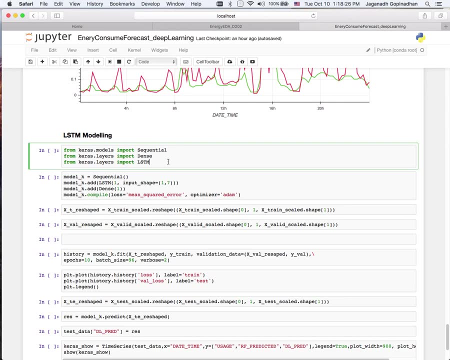 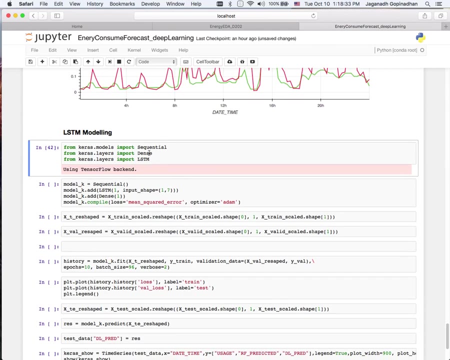 will just focus on the practical aspect. so i'm using a keras with tensorflow, not with gana or or cmtk- yes, with tensorflow- or google tensorflow library. i just used a tensorflow library, but i'm just importing the basic basic library, such as the sequence, dense and lstm fpis here. 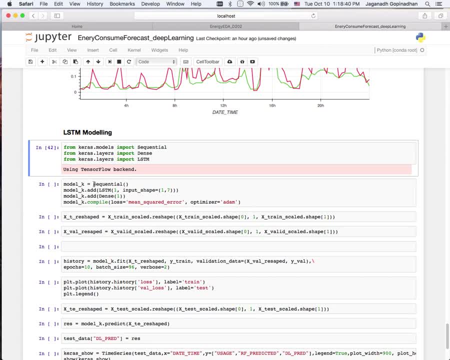 so this part, i'm defining my model. so then i'm defining a sequential model. i'm adding an lstm with an input trait of one and same one and one and seven. that means one dimension and seven attribute is there. i'm adding a dense layer here and i'm using the loss as a mean square error and 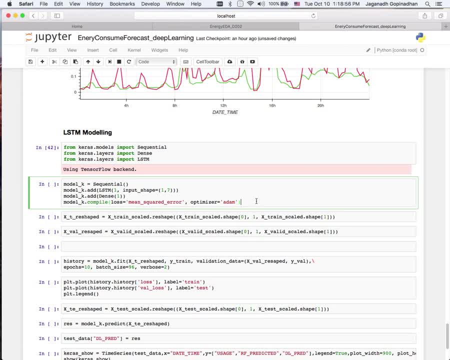 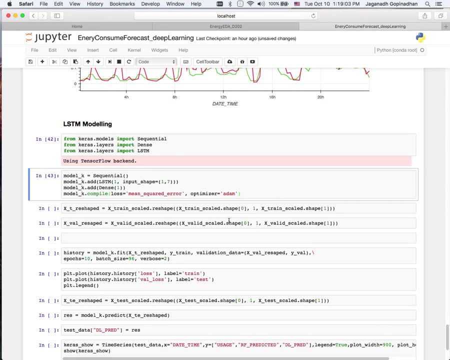 an atom optimizer is being used here as my optimizer. so this is a very basic, very, very elementary model, lstm model: here you can be more creative and you can add a start lstm layer after this particular one. you can add an lstm with stateful. you can add a stateful lstm. 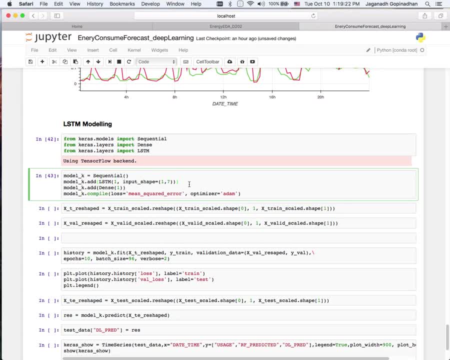 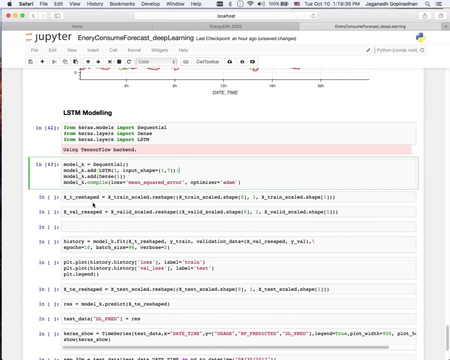 or or non-stateful lstm, etc. here, and you can make the model more robust, but for the time being, let's try to make make this as very simple. so the data which we already created, the, the scaled data, is basically in two dimensions. so what the lstm model expect is is a three-dimensional data. so i just 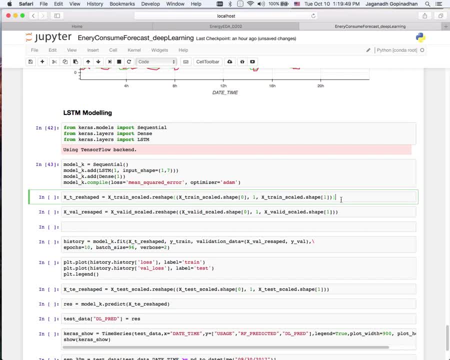 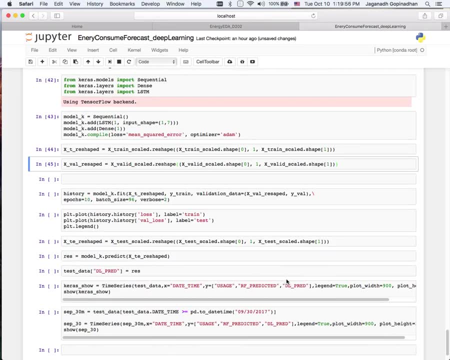 tried to make it as a as a three-dimensional data. so my training data and validation data, i'm just writing the shape in the three-dimensional. later i will make my validation data also to be a three-dimensional one. okay, so i'm trying to fit the model and i'm supplying 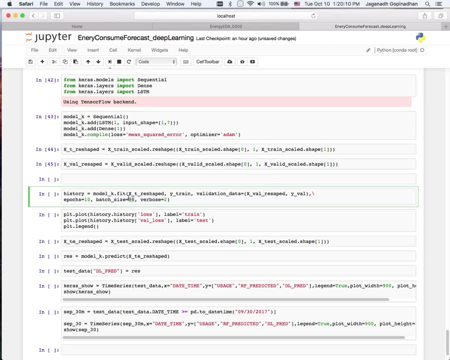 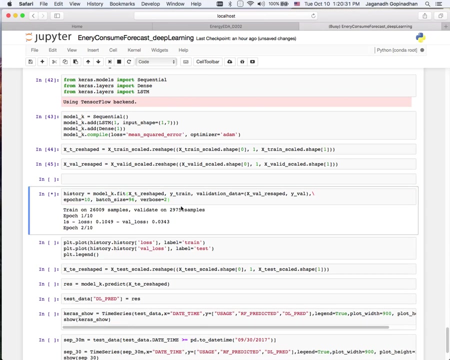 my validation data here and i'm saying that batch size is equal to 96, and just run 10 epochs and and just run the model, so in a single batch it will feed 96 observation to this model and it will be a. So let's run the model process here, okay, so this is running. you can see that it's. 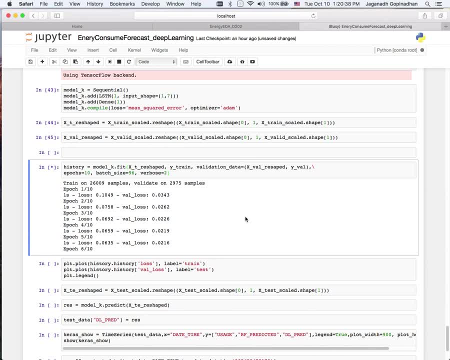 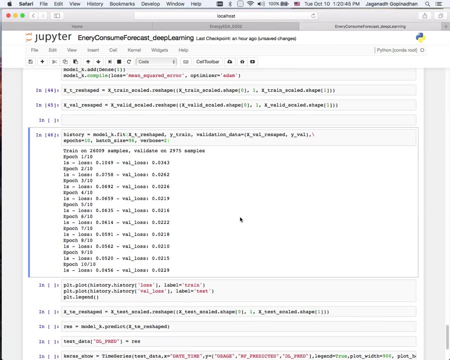 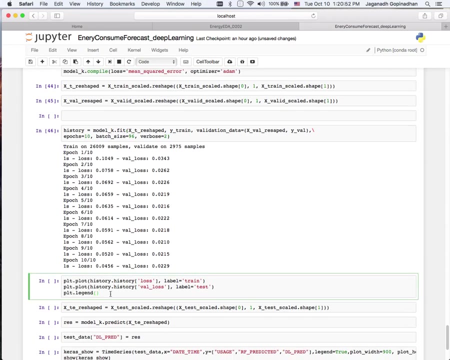 running pretty fast, so it's completed. 5 epochs, 6 epochs 7, 8, 9 and 10, okay, so now our training process, or the model building, is completed in 11 seconds, I would say, and. 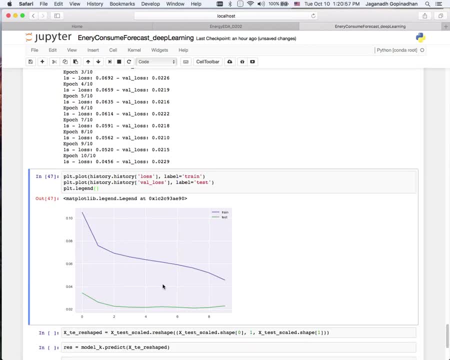 let's try to see how the training and the validation loss looks. okay, you can see that the training loss is slowly decreasing, and so the test loss, but we can see that it's almost getting stuck and under here. in 10 epochs maybe we might have made a wild wise. 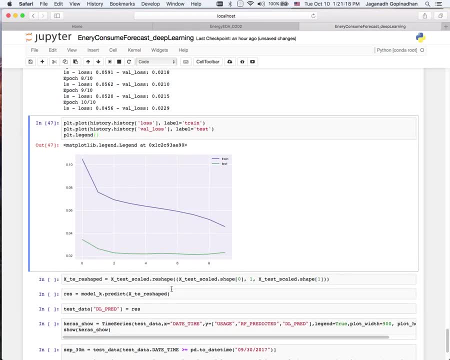 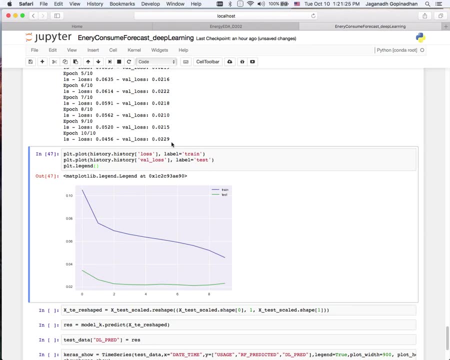 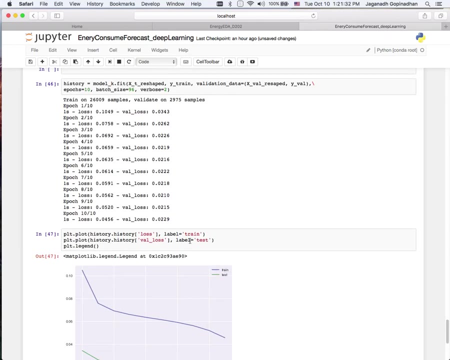 choice, believe. okay, So we can see that the training, the training loss was 0.64, and the validation loss was 0.29,. yeah, from the given data and given hyperparameter again in the case of this, 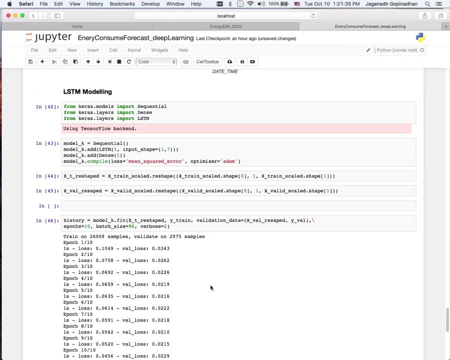 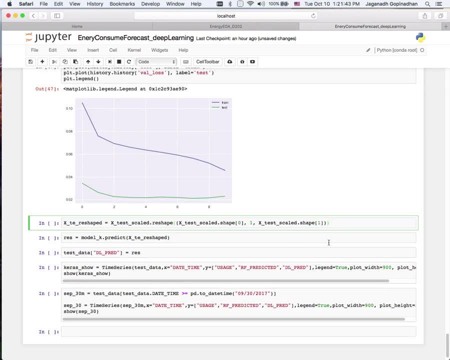 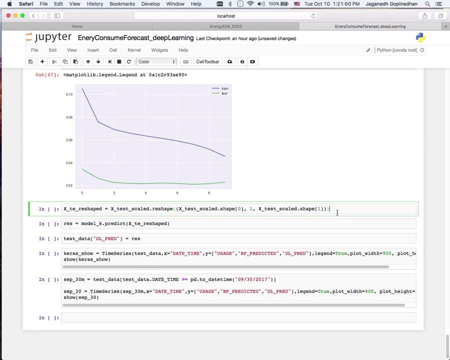 model. also, I didn't do much of a hyperparameter tuning, so we can say that this is just working model, not a robust model. so we have to do more hyperparameter tuning to make the model more efficient. So we can say that this is just working model, not a robust model. more robust, robust and 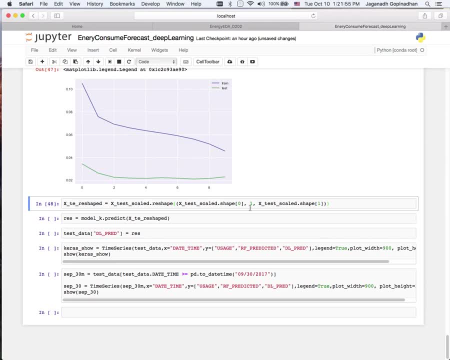 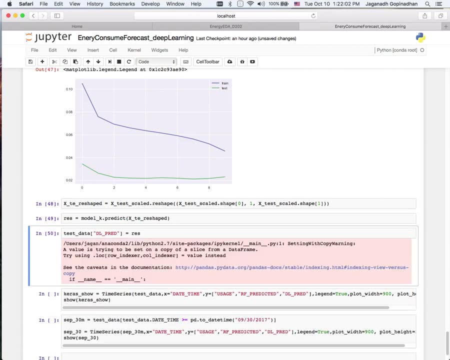 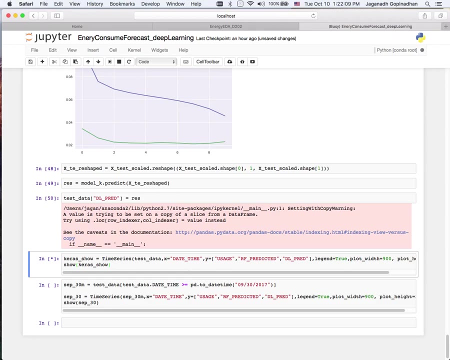 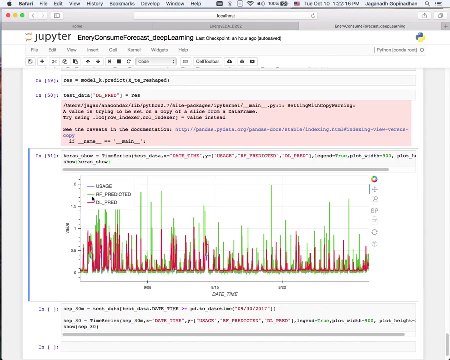 efficacious. so just reshaping my testing data and I'm predicting the data. so the prediction happened and I'm appending that into my test data, my test data. so let's try to see the prediction here. So I'm just plotting the actual usage. actual usage is blue line, the random product prediction. 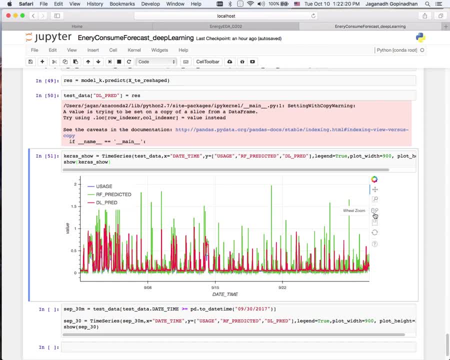 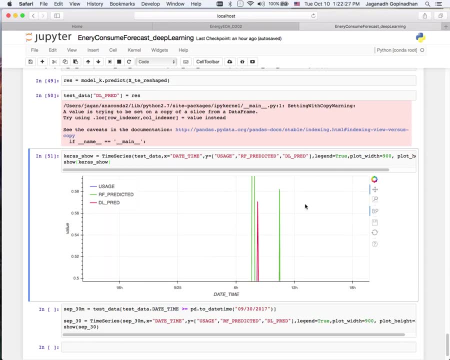 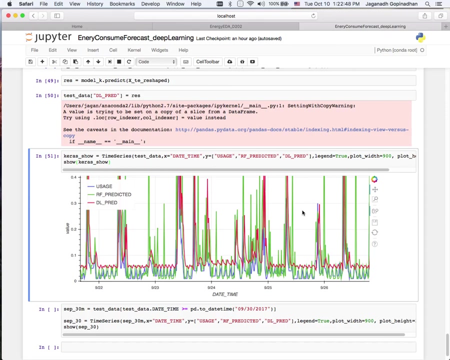 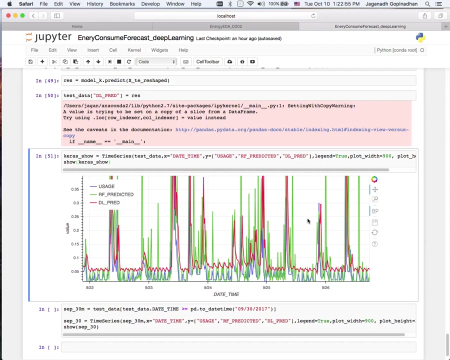 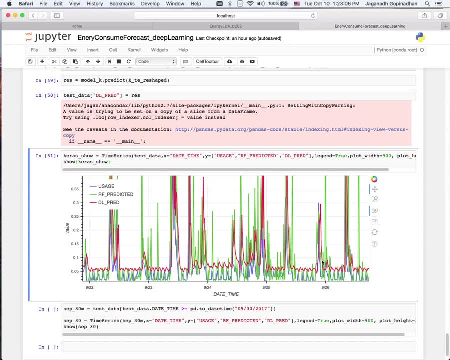 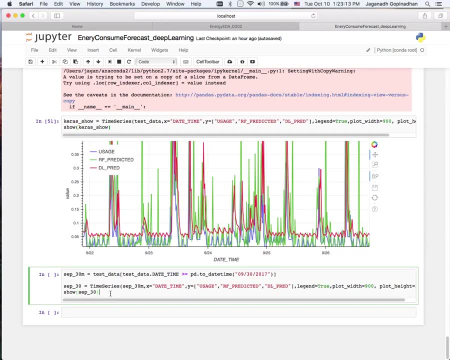 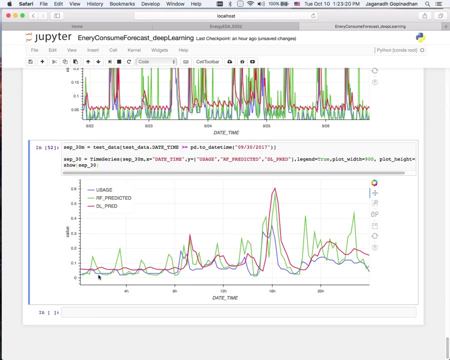 means we may have to enhance the model a bit more, better. So let's take a very, very closer look on how, on how we predicted in the case of 36.3% September 2007, and you can see that, rather than like predicting all these, 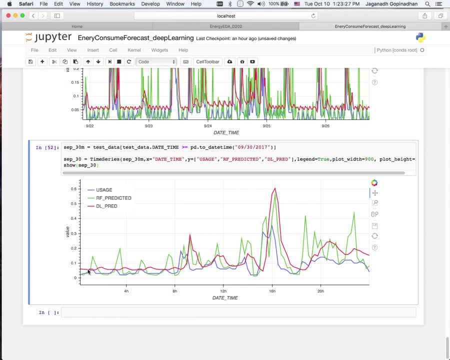 peaks. my model predicted all these peaks as a very steady one, that is, 0.05 or 0.5 kilowatts throughout the day, but the the peak in the morning was being almost explained like this, almost in the closing post or closed prediction and in: 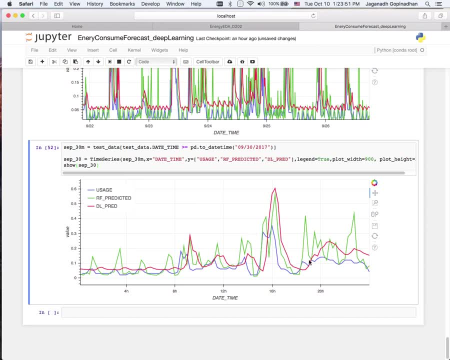 the afternoons and pretty much in the in the evening or almost in the late nights also to be able to come there. maybe a bunch of additional hyperparameter tuning may help us to make this met the model pretty much better. so in this time we are going to talk about the hyperparameter tuning and we are going to 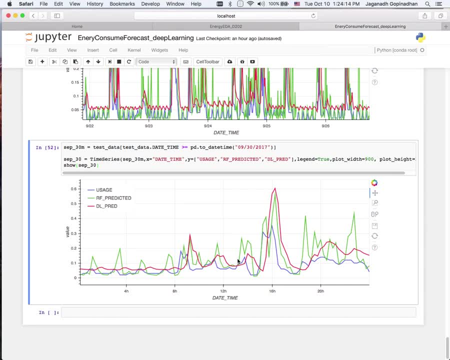 talk about the hyperparameter tuning and we are going to talk about the time series forecasting. so I just showcased a couple of very elementary techniques, but I just give a hint on how we can create additional features from the time series data and, as a library- Pandas is a great library- to create such 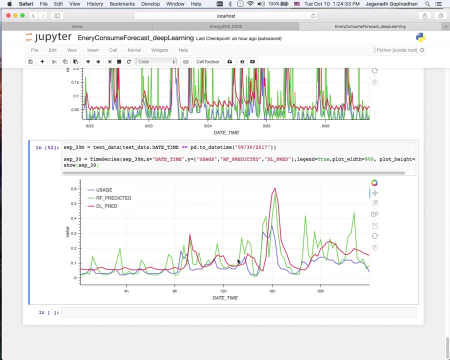 additional features there and you can bring additional data from the NOAA website, etc. to bring extra data and make your forecast more and more better. and at the same time, I just showcase how we build a query baseline model with random forest regression technique. and then we built an LSTM- very simple LSTM model. yeah, but both of our models are not so. 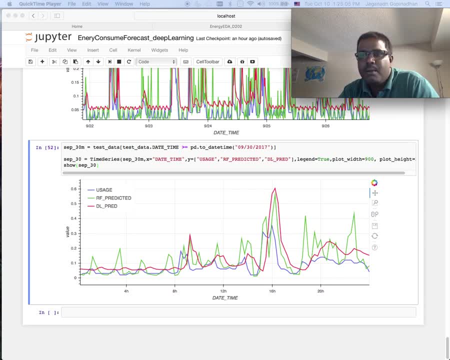 great in terms of its prediction capability, but it serves as a basic tutorial on how we can create an LSTM model. so in some of the next version I will come up with a stacked- stacked LSTM models and LRNN models or GRU models in time series forecasting. I hope you will be able to get a quick. 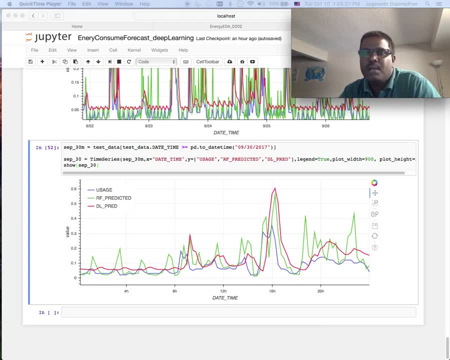 glance on it. I'll be uploading this IPath notebook in my github and in the Anaconda libraries for your future reference. the data set will be also be available there. you may find another alternative data sets in the UK government's open data website for for half-hour energy consumption. yeah, the principle doesn't. 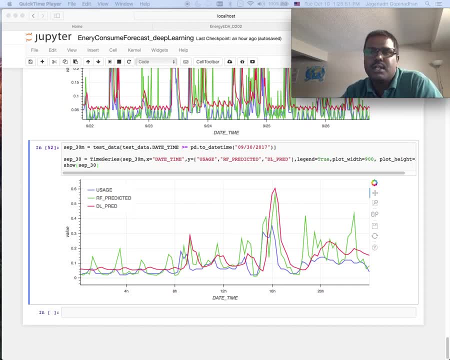 change there. here I am getting around 15 minutes interval energy forecasting, 15 minutes interval energy data. the UK we have the smart smart meters are measuring 15 minutes. if you're living somewhere around around pan-asian regions you may have Singapore or some other countries give again.